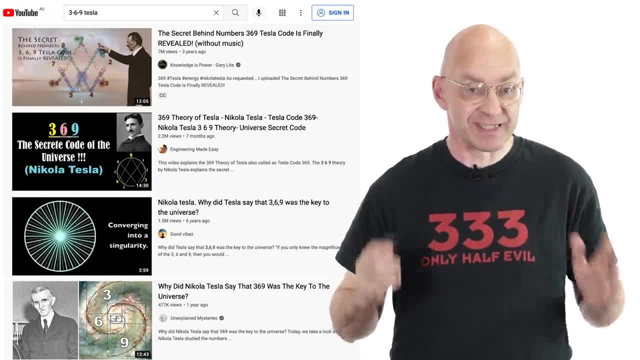 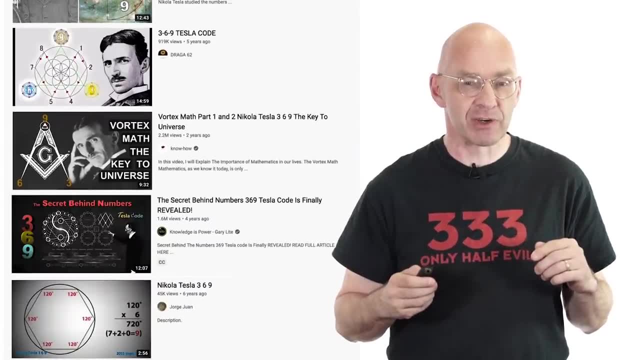 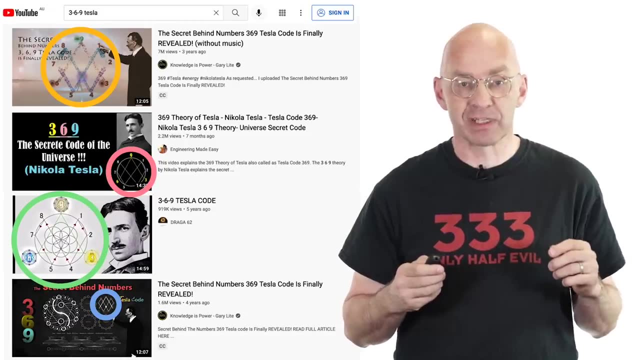 369 tesla on youtube: a pile of seriously viral videos. 7 million views- Not bad, huh. A lot of these videos feature a curious diagram in their thumbnails. This diagram is usually referred to as the vortex and is one of the main topics covered in these videos. 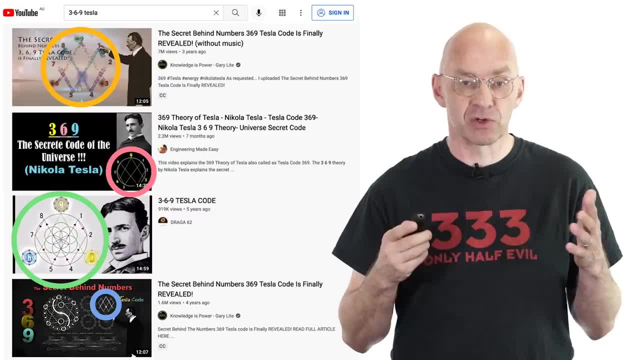 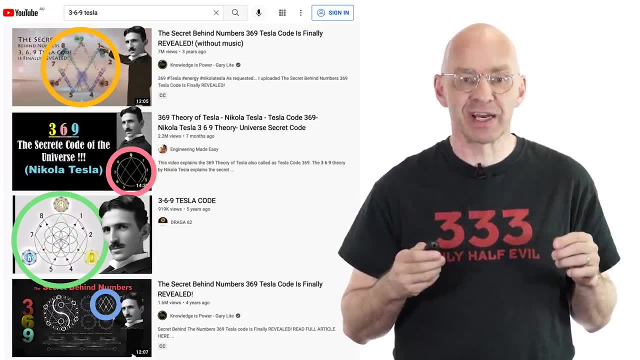 You've all heard of Nikola Tesla, the genius inventor of the tesla coil and other early electrical devices. right, The tesla car, that tesla. But did you know that tesla also had a host of idiosyncrasies centered around the number three? For example, tesla would walk three times. 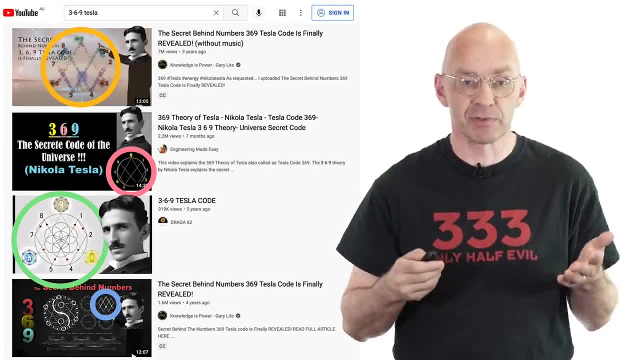 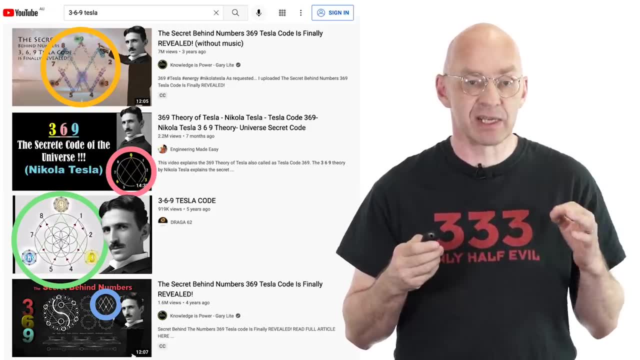 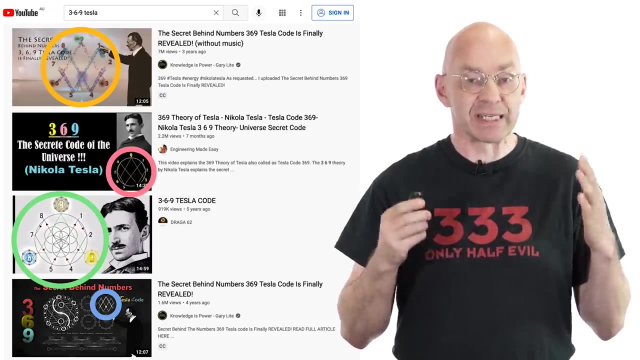 around a block before entering a building. He would only stay in hotel rooms with a room number divisible by three, and so on. In general, he was convinced that the numbers three, six and nine hold the key to the universe. According to the champions of vortex maths, the vortex is that key. 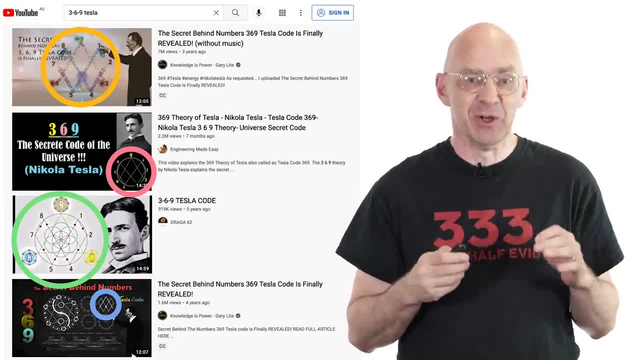 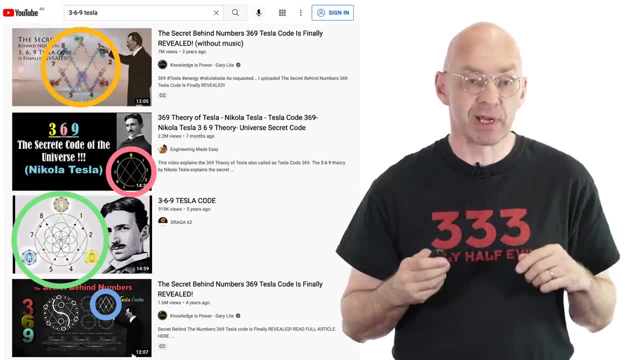 That sounds a bit nuts, But, as I said, I'd never heard of vortex mathematics, and so I was curious to find out more. And seven million people can't be wrong, right? Also, although vortex math was new to me, I'd already stumbled across the vortex diagram. 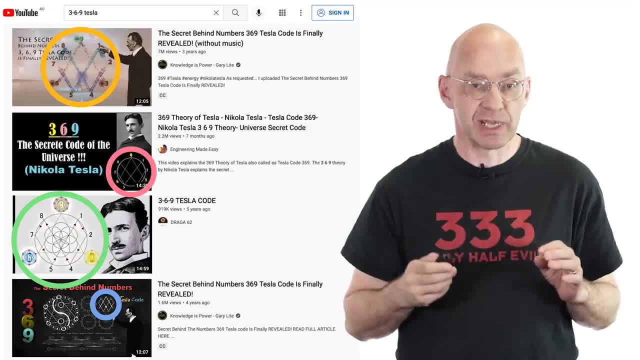 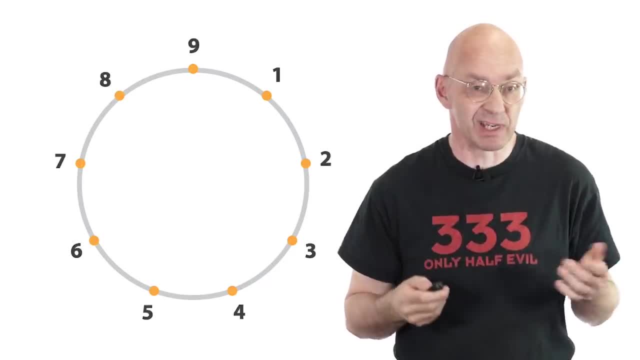 before, in a different context. Anyway, our mission today is to have a closer look at the vortex There. nine points on a circle labeled one to nine, innocent enough. Then there's this infinity-shaped loop connecting six of the points. The remaining three points. 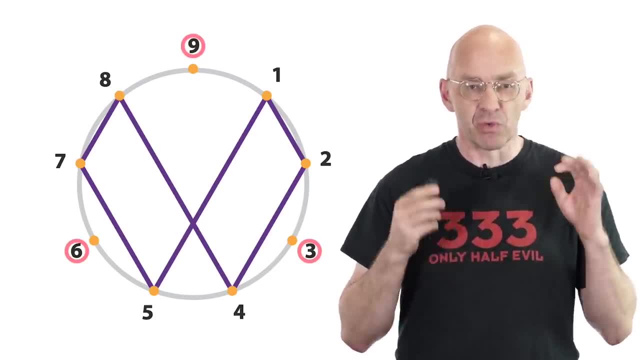 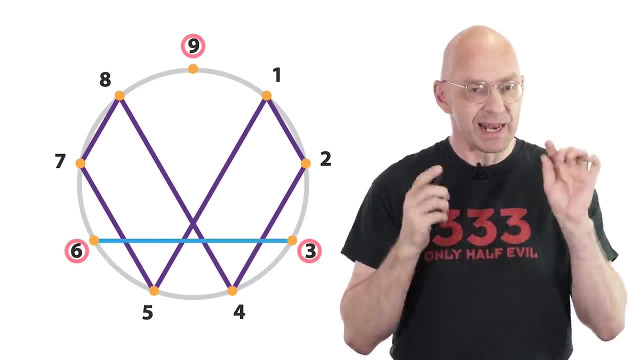 three, six and nine form an equilateral triangle and, depending on which video you watch, some extra lines get added, like this, Or like this, Or like this. The last version of the diagram is the one that I have been familiar with for many years. It's part of a famous sequence of diagrams. 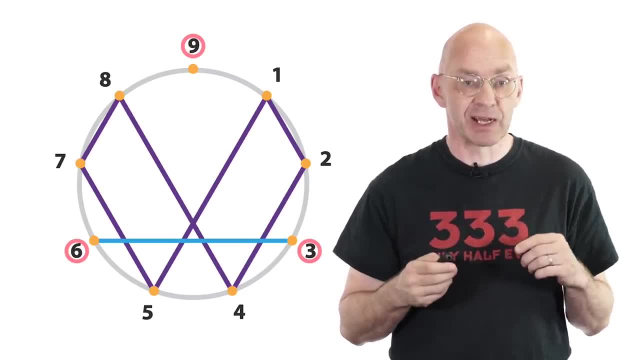 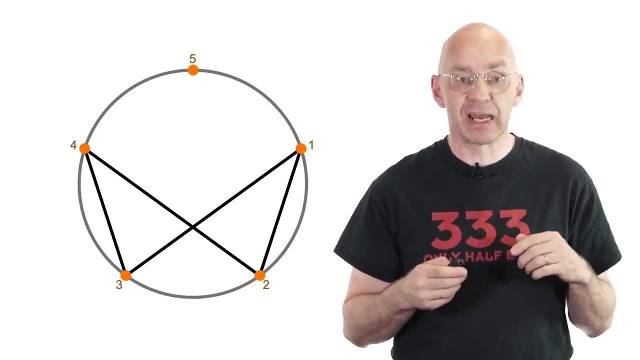 one diagram for each positive integer. This sequence of diagrams starts out like this: That's a diagram for one, for two, for three, for four, for five, and so on. Nine, that's the vortex, and then things continue like this: 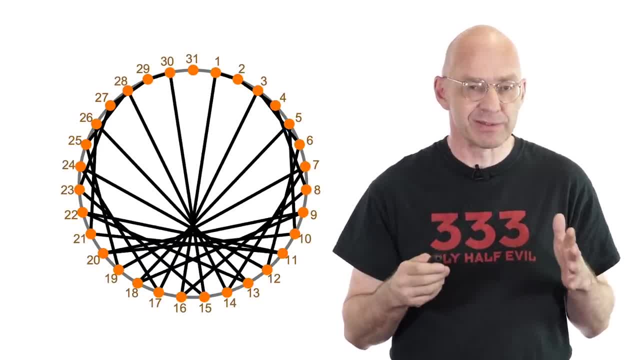 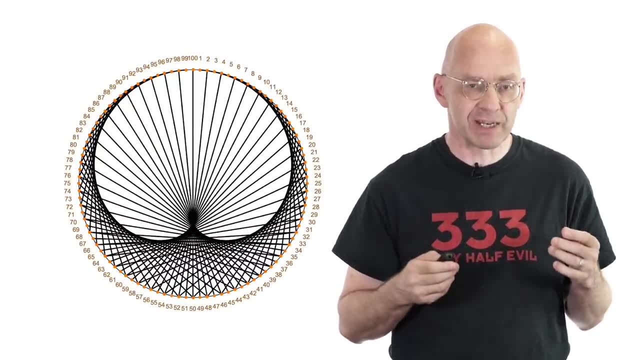 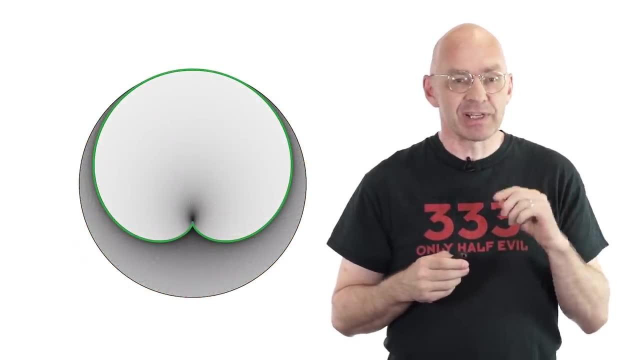 Okay, does this all look a little familiar? No, Well, then let's keep on going. Okay, what's going on here? Well, I'm sure a lot of Mathologer regulars will recognize these diagrams and the pretty curve that is starting to materialize. We already encountered these diagrams. 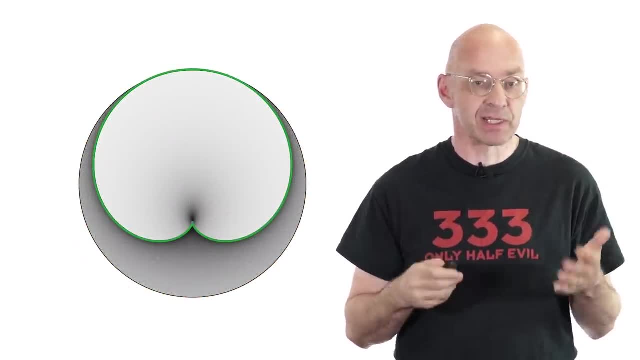 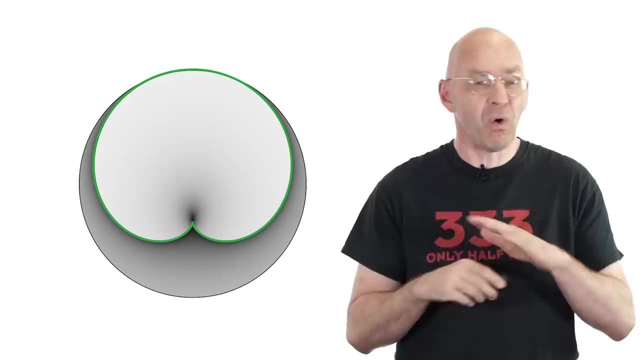 in the Mathologer video on the times table, the Mandelbrot set and the heart of mathematics. the curve is called the cardioid, the mathematical heart curve. It pops up in mathematics and nature all over the place. For example, it's the curve you get when you roll a circle around another. 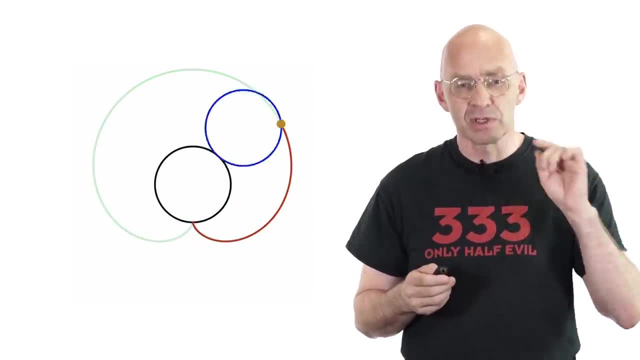 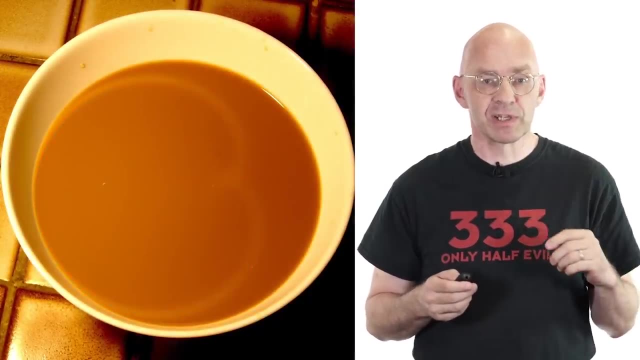 circle of the same diameter like this. It's also the curve that you often see in cups on Sunday days, Okay, and it's the curve that takes center stage in the Mandelbrot set. The Mandelbrot set. there it is. 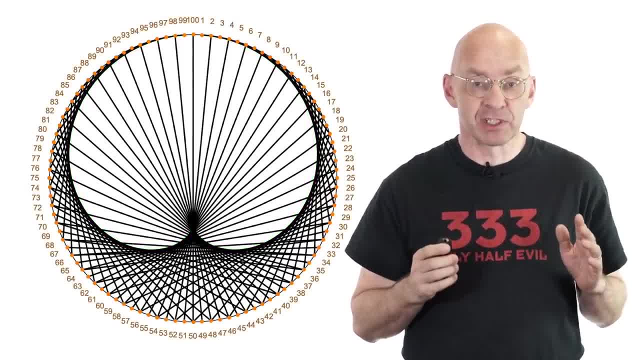 Actually, there's more, much more. Every positive integer does not only give rise to one of these cardioid-infused diagrams, but to a whole family of line diagrams, And a lot of these extra diagrams are also incredibly complex and beautiful. Here are just a few examples. 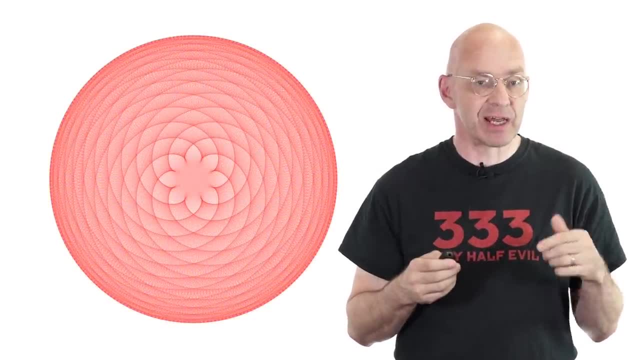 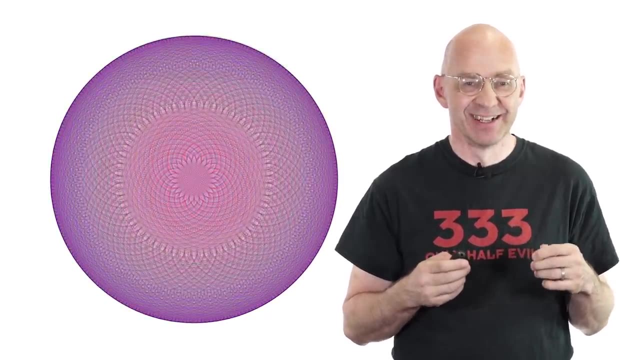 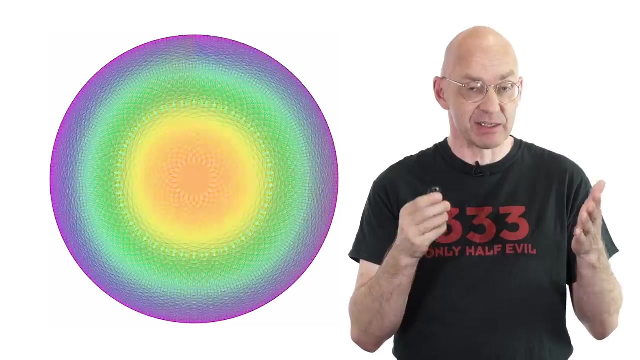 Pretty spectacular, isn't it? It gets even more impressive when you color the segments in the diagrams according to their lengths. Whoa, not bad, huh, But that's enough pretty pictures. We're on a mission, remember. Our goal is to make sense, mathematical sense. 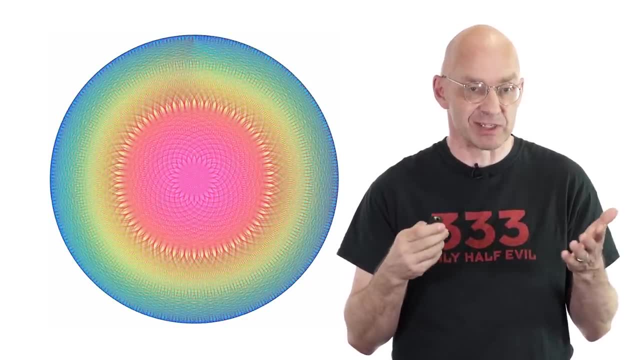 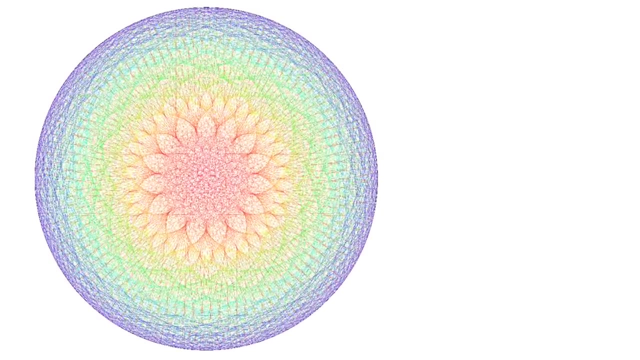 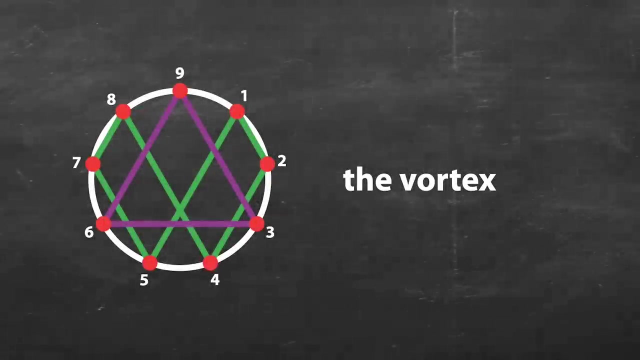 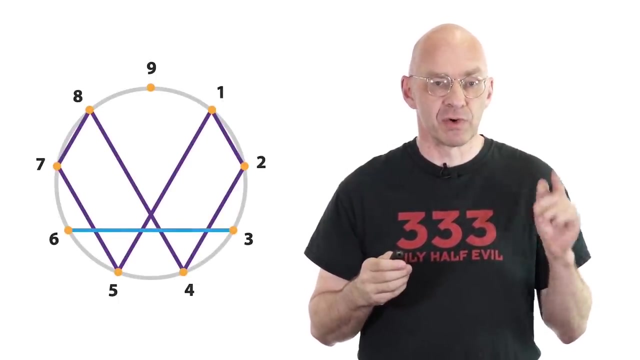 of the vortex, Which includes making sense of its mysterious relatives, Interested? Well, why wouldn't we be right? So let's get going. Okay, all the tesla code videos I mentioned earlier introduce the vortex to an entirely new one. the vortex in essentially the same way. Here we go. Start with the powers of two. 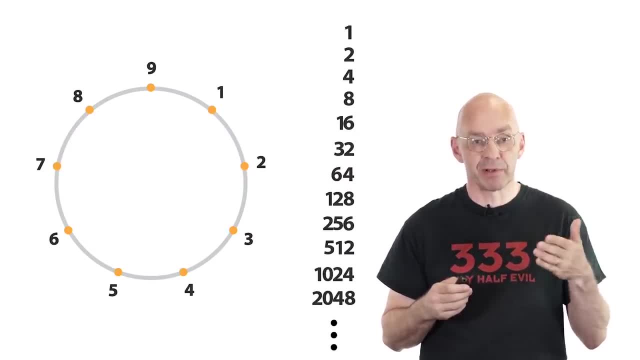 So begin with the number one, and then every number is double the number before it. Next, for each number in this table, we calculate its so-called digital root. For this we keep adding the digits of a number until we end up with a single digit. For example, in the case of 128, the sum of the digits is 1 plus 2 plus 8 is 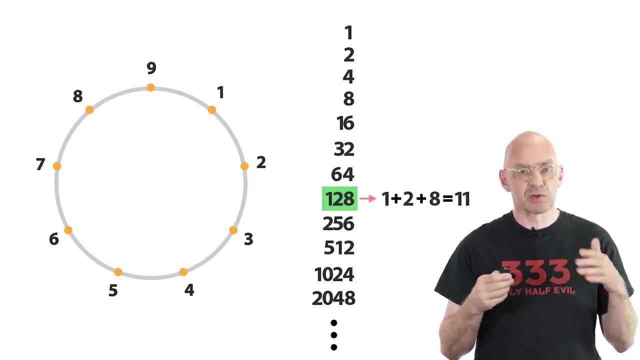 11.. Now, 11 is not a one-digit number yet, and so we keep on going. 1 plus 1 is 2, and so the digital root of 128 is 2.. Easy, right Now let's do this for all the. 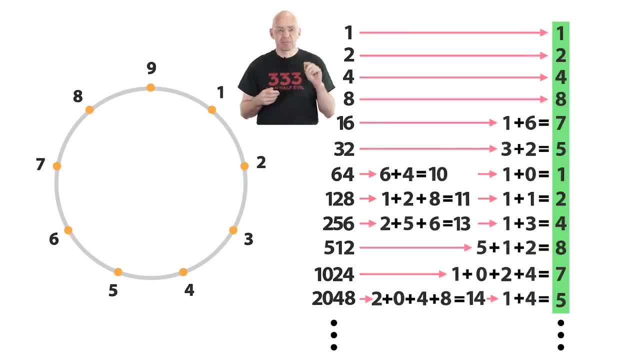 numbers in our sequence There. Let's string up those digital roots on the circle First: 1, 2, 4, 8, 7, 5, 1, 2,, 4, 8, 7.. In fact, we'll keep on going like this. 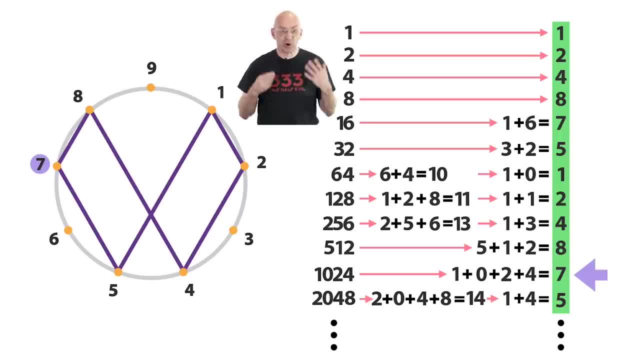 forever: 1, 2, 4,, 8,, 7, 5, 1, 2, 4, 8, 7, 5 and so on. over and over. Pretty cute And also pretty surprising. right Now, instead of doubling, let's look at the. 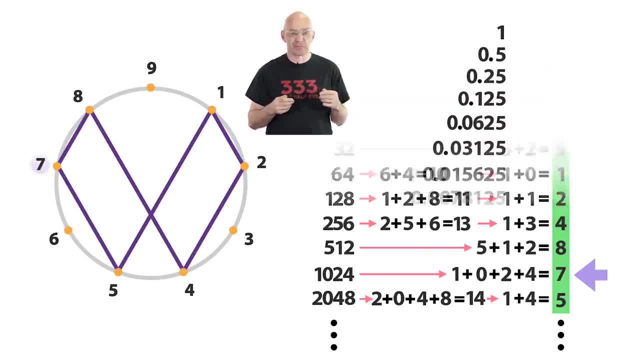 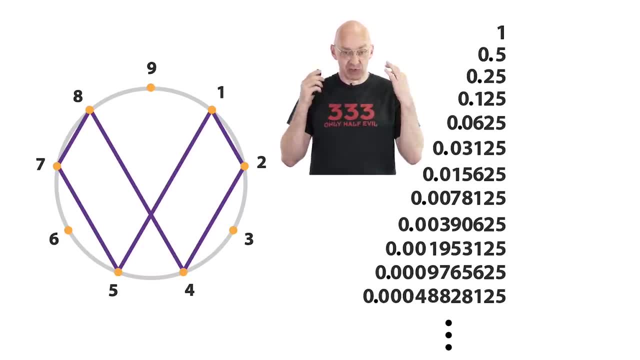 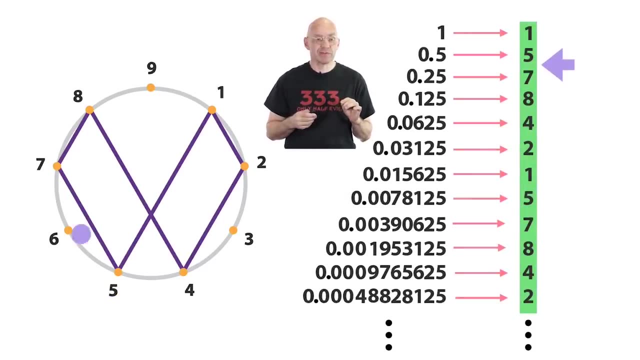 sequence we get by halving Again, starting with 1.. 1, 1 half is equal to 0.5, 1 fourth equal to 0.25, and so on. Let's calculate the digital roots of these numbers. Looks familiar, right? Let's check what happens on the circle 1, 5, 7,, 8, 4, 2.. 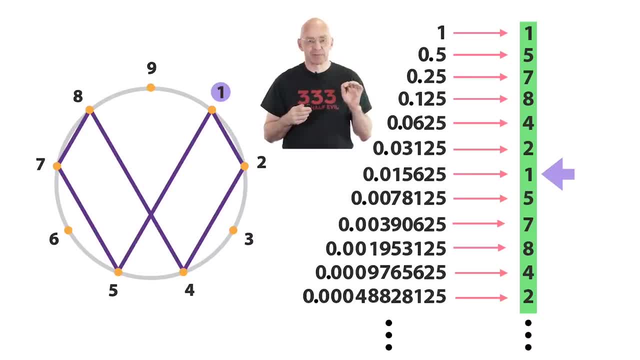 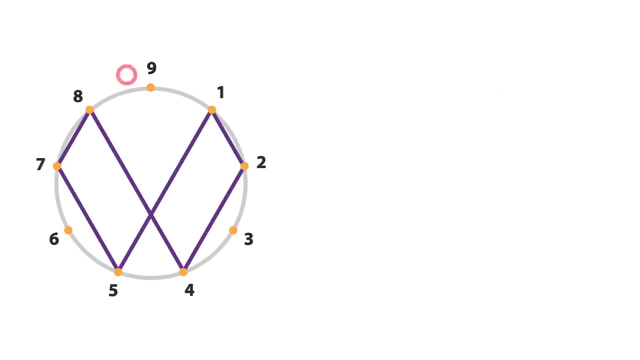 The same digital roots as for doubling, Just in reverse order. Again, repeating forever and ever after, Also pretty cute, right? But notice that there are three numbers that never get visited: 3, 6 and 9.. Tesla's 3, 6 and 9.. Whoa, At this point of the discussion, the absence of Tesla's 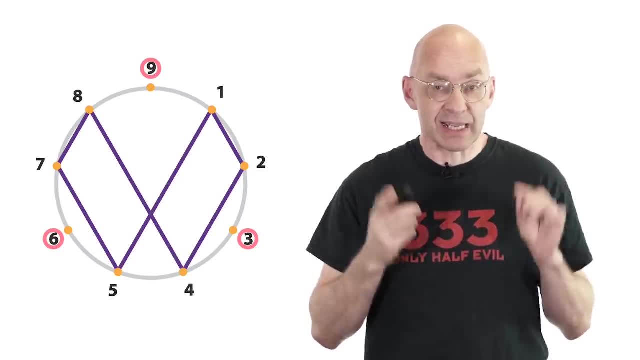 3, 6 and 9 from the cycle is usually interpreted as a telltale sign that we're dealing with some sort of divine message, some secret code, the powerful key to the understanding of the universe that Tesla will serve. What are we raving about? Well, maybe, I have to admit that I'm not quite able to follow. 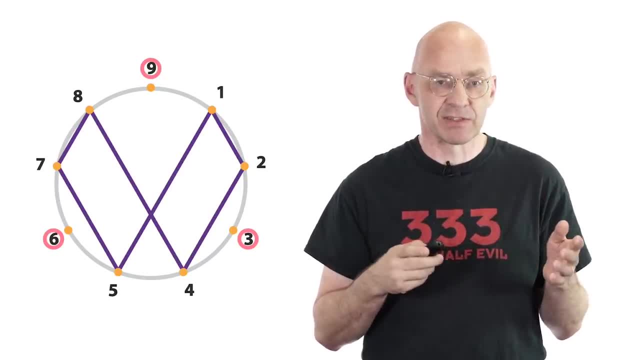 the line of reasoning here. However, judging by the zillions of likes these videos attract and their enthusiastic comments, pretty much everybody else watching appears to be in awe and fully on board with what's going on here. Must be just me, I guess. 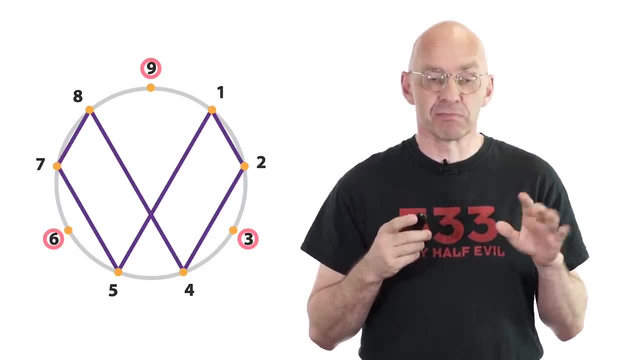 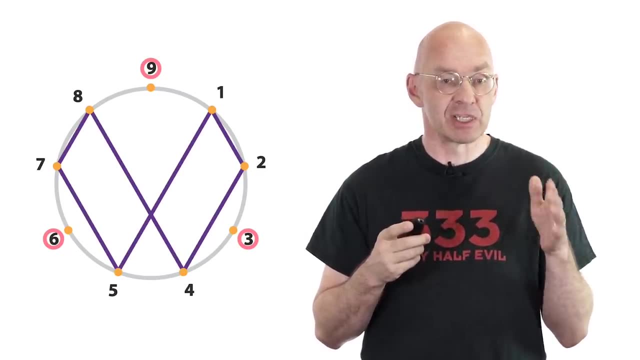 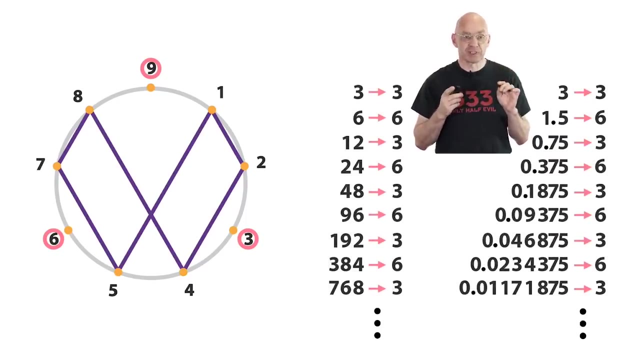 Of course, there is more evidence that the vortex is the key to the universe. Much more. Now we are told to look at what happens when we keep doubling and halving, starting with 3.. Whoa, The plot thickens. Both. for doubling and halving, the digital roots alternate between 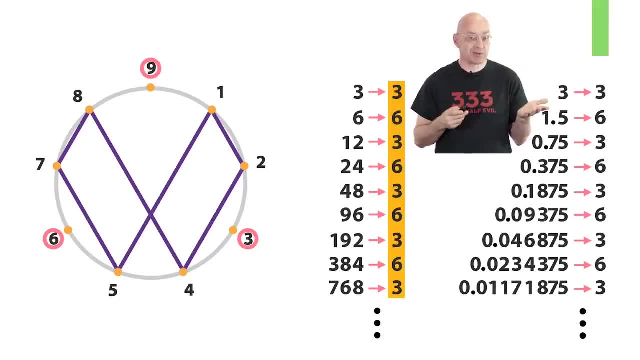 3 and 6.. There 3, 6,, 3, 6,, 3, 6 and so on, And there 3, 6 and 3, 6 and 3, 6, again The 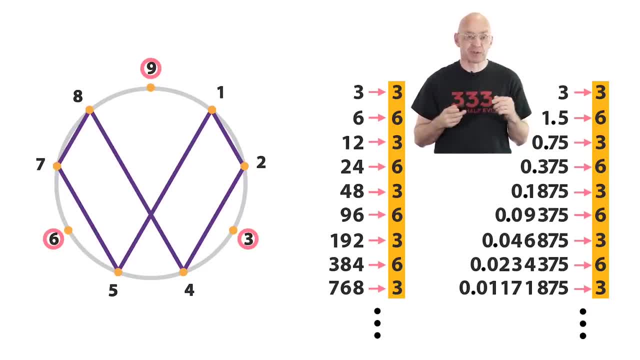 alternating 3,. 6 then corresponds to a line between those numbers in the diagram, Definitely key to the universe, right? And what about the 9?? At this point in time, the makers of all those videos get really excited. We get all 9s- Amazing. 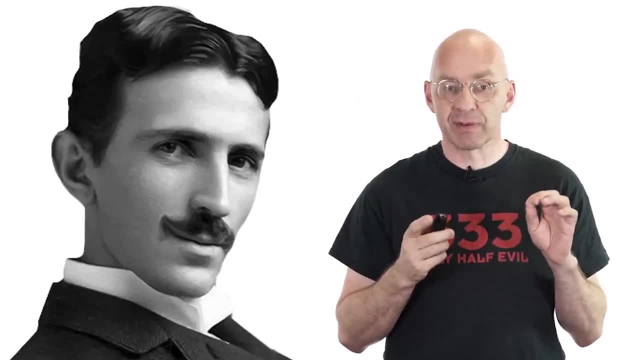 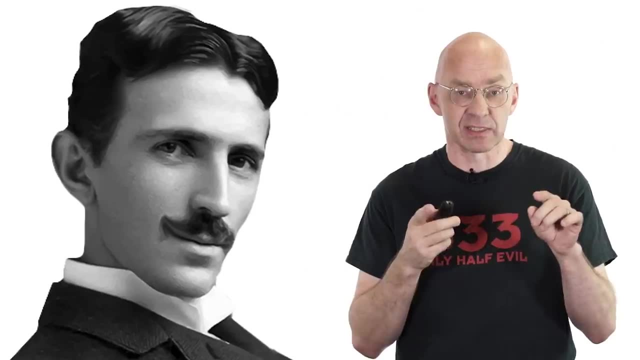 To round things off, it's then also pointed out that a lot of the other famous numbers in maths have digital root 9.. For example, 360, 180, 90, 45 degrees, the number 666, this guy here, All those numbers have digital root 9.. Key to the universe. How can it be? 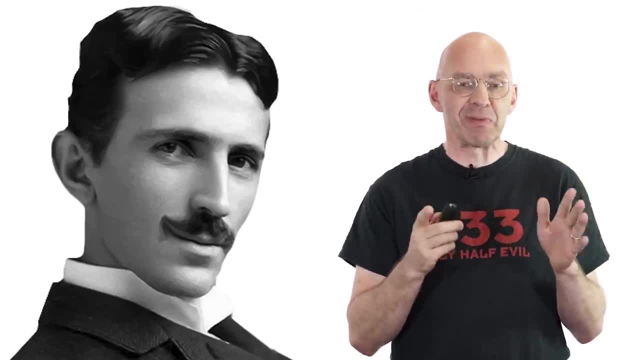 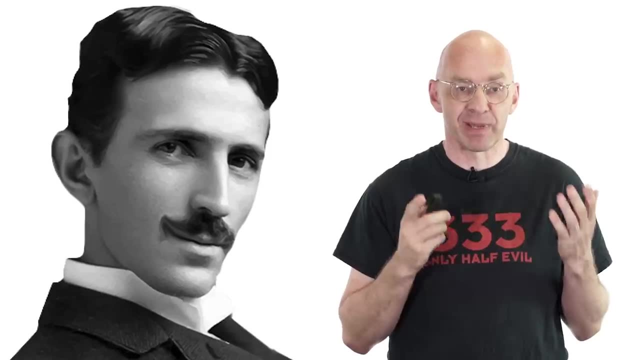 otherwise, Ok, ok. I can see plenty of you screaming at your computers trying to get a butt in. And yes, of course you are correct. Everything we've seen so far has a fairly clear line. Everything we've seen so far has a fairly simple mathematical explanation. Part of 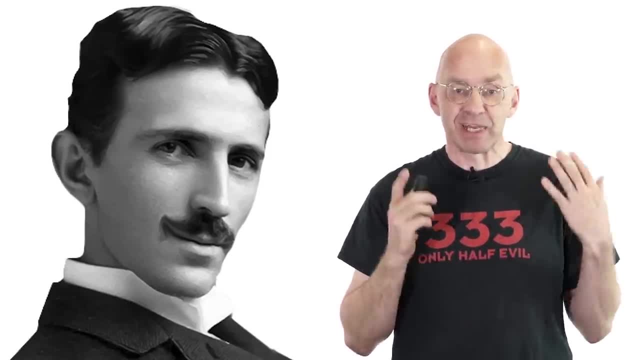 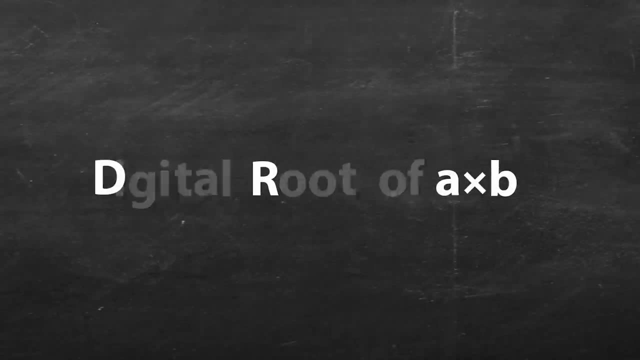 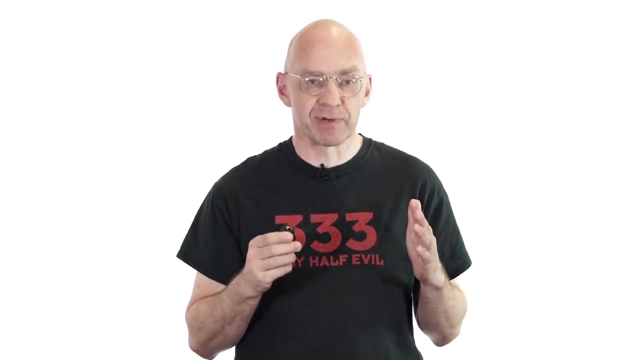 which just about everybody has been exposed to in school. An explanation that, by the way, never gets mentioned in Vortex Maths videos. Funny that Right Where in school mathematics do you add digits over number? Remember Divisibility tests. 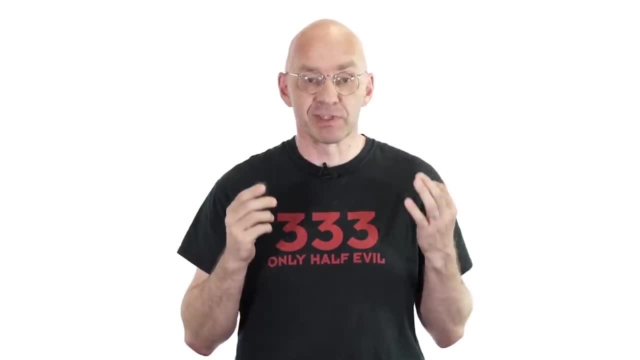 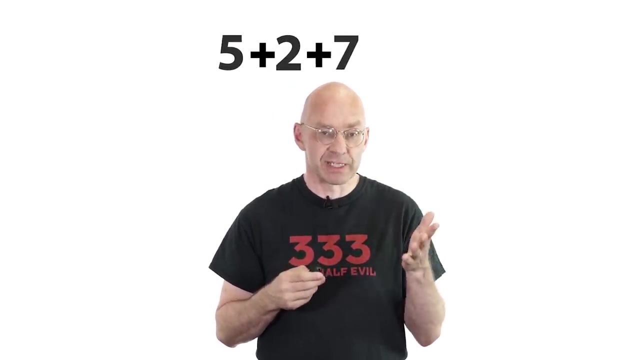 If you want to find out whether or not a number is divisible by 9, you just add its digits and check whether this digit sum is divisible by 9.. That's how it's usually taught in school. As a refresher, let's do an example: 527.. Ok, 5 plus 2 plus 7 is 14 and 14 is not. 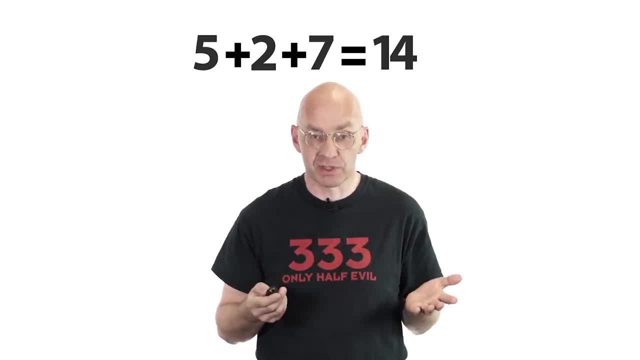 divisible by 9, and so 527 is also not divisible by 9.. Well, of course, if that works, then you can repeat, adding the digits until only the digital root is divisible. And then, very simply, a positive integer is divisible by 9, exactly if its digital root. 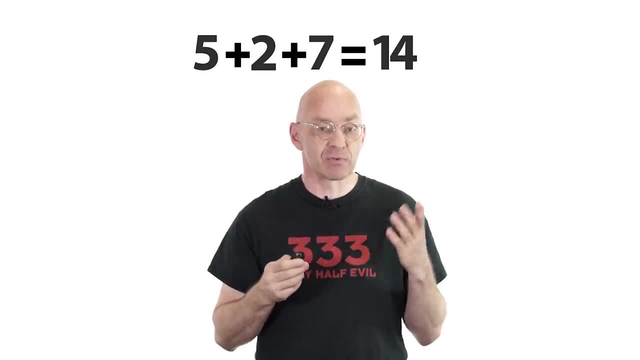 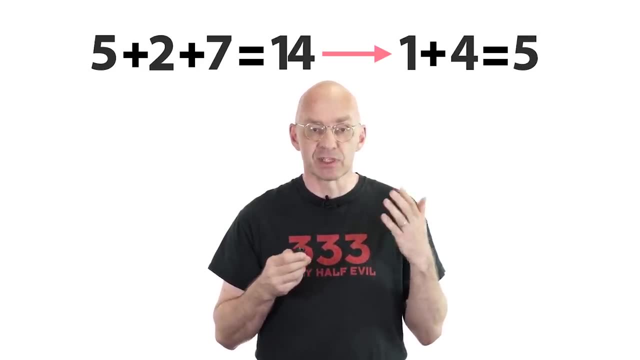 is 9.. In our example, the digital root is 1 plus 4 is 5.. So the digital root is not 9.. And we come to the same conclusion as before: 527 is not divisible by 9.. In school they 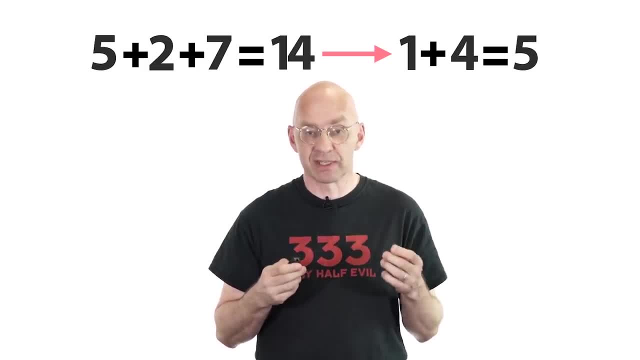 usually don't teach this simple digital root extension of the standard divisibility test for 9.. Of course they should teach this in school, but they don't. In fact, what they should also teach is that IF the digital root of a number is NOT equal, 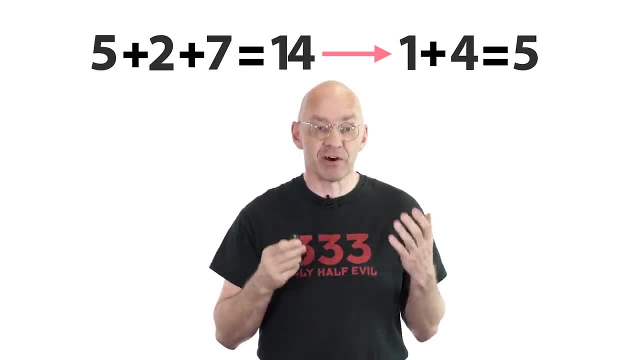 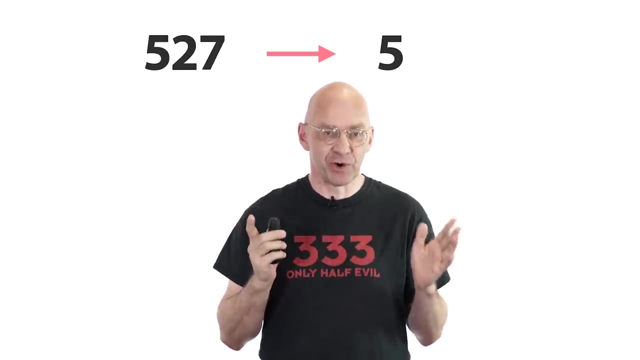 to 9, then this digital root is simply the remainder of that number on division by 9.. Nice, huh. So the remainder of 527 on division by 9 is our 5 up there Great. Now, just out of interest. were any of you out in viewer land taught this remainder extension in school? 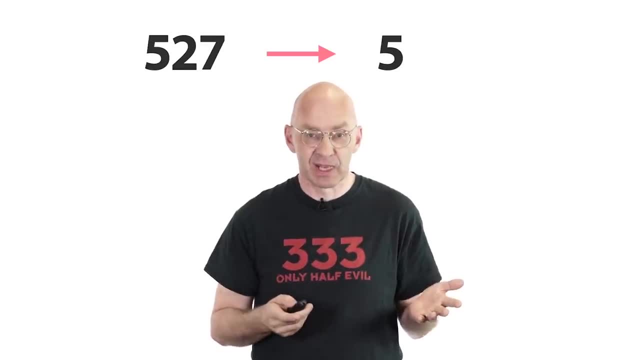 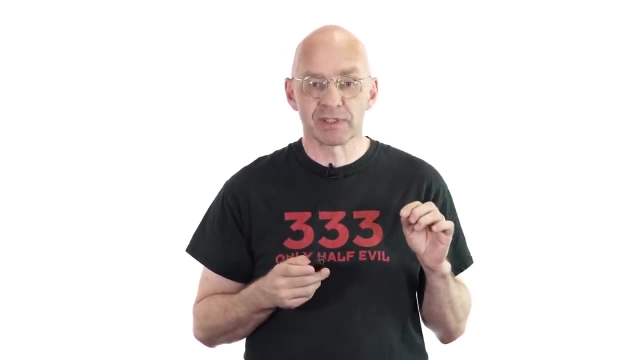 Anyway, very much worth knowing and teaching, don't you think? I'll show you the simple proof for all this in a little while, but for the moment, let's keep on going To explain what's really going on with all that vortex maths I need to remind you of. 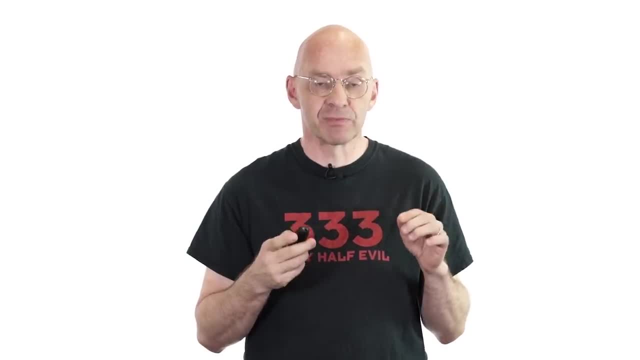 two more super important properties of remainders on division by any number, as well as the digital root's counterpart of those properties, in this special case of 9.. Nothing scary, really, just primary school level maths promise. What are those properties? Well, the first property is that the remainder of the SUM. 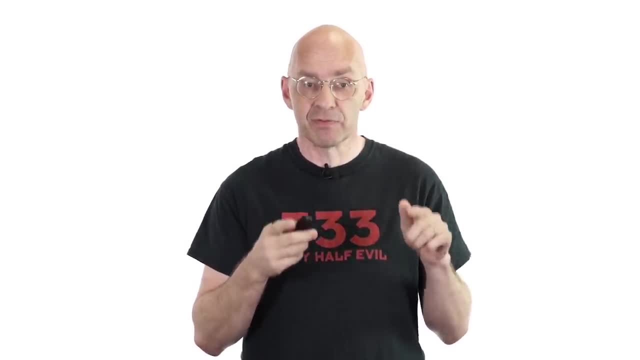 of two numbers equals the remainder of the SUM of the remainders of the two numbers, and the second property is the exact corresponding statement for products of numbers. That's all a bit of a mouthful, but a quick example will make it clear what I mean. and at the 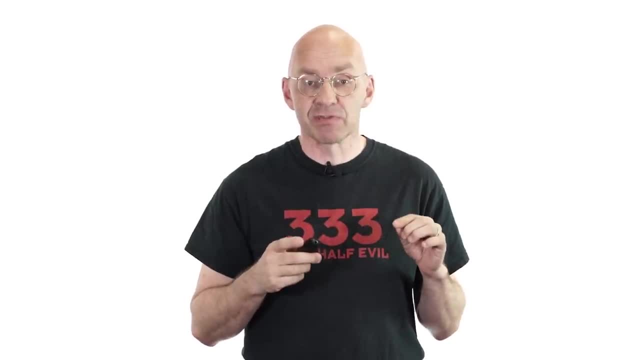 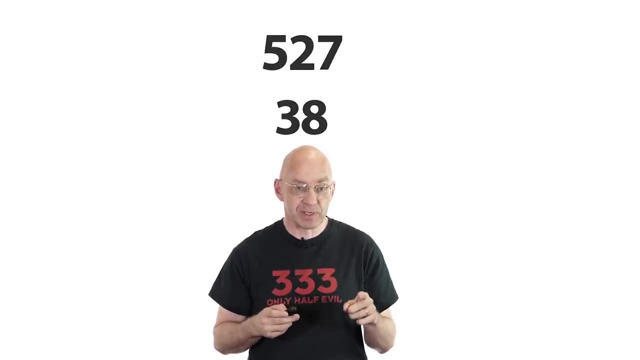 same time show you why it works. Ok, let's just stick with division by 9 and let's pick two random integers: 527 and 38. Now, 527 is 9 times 58 plus 5.. You can check this And therefore, when you divide 527 by 9, you get a remainder of 5.. 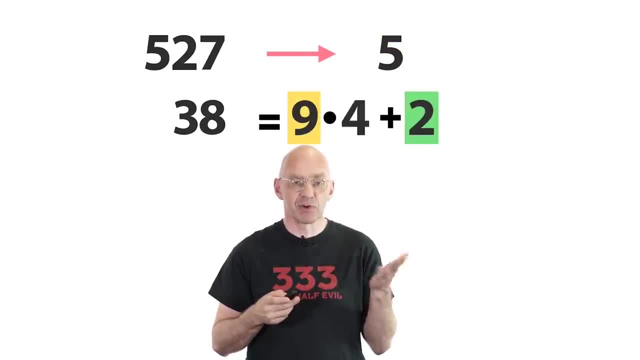 Similarly, 38 is 9 times 4 plus 2, and so the remainder is 2.. Ok, what if you are also interested in the remainder of the sum of 527 and 38?? Well, of course, you can just add the two numbers, divide by 9 and this way find the remainder. 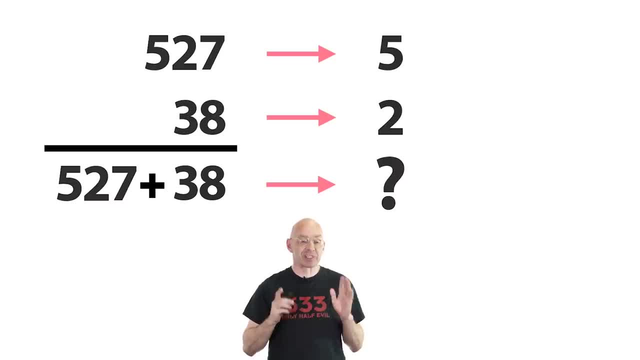 Yes, you can do that, but there is a much, much quicker way. Have a look Again. 527 is 9 times 58 plus 5 and 38 is equal to this. Ok, adding the stuff on the right, we get this. 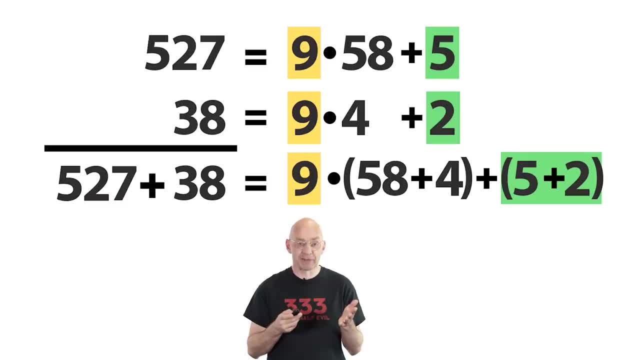 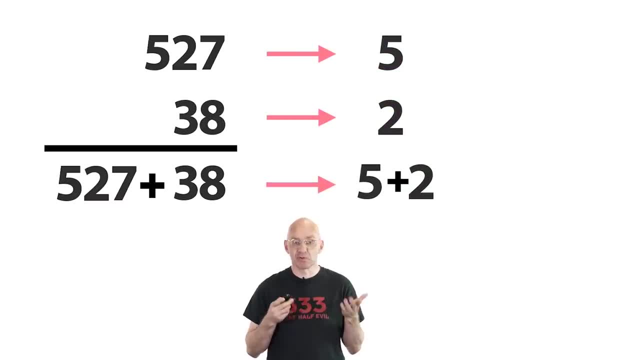 So what this shows is that the remainder of the sum on the left is simply the sum of the original remainders, 5 and 2.. 5 plus 2 is 7, and so the remainder is 7.. Super simple, right? Well, mostly, but sometimes we have to deal with a little hiccup. 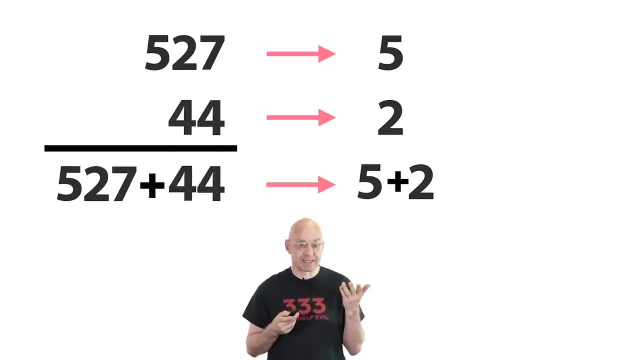 For example, if we replace 38 by 48. Going up by 6, the 2 on the right becomes an 8. And 5 plus 8 is 13, which is greater than 9, and so not one of the possible remainders. 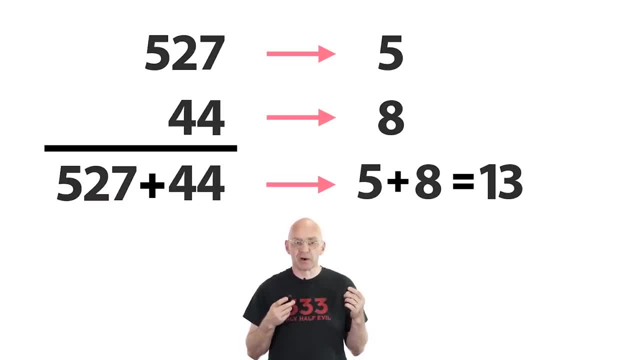 on division by 9.. But that's easily fixed. What's the remainder of 13 when you divide by 9?? Well, 4, of course. This means that the remainder of 527 plus 44 on division by 9 is 4.. 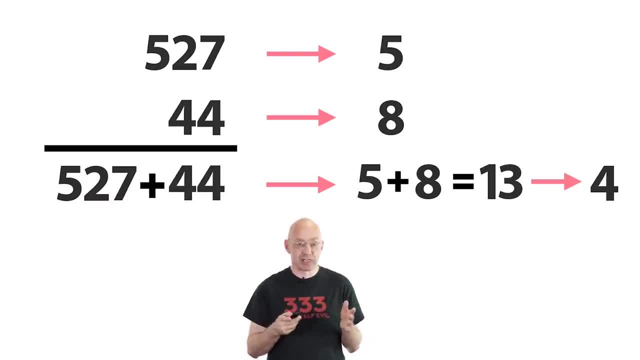 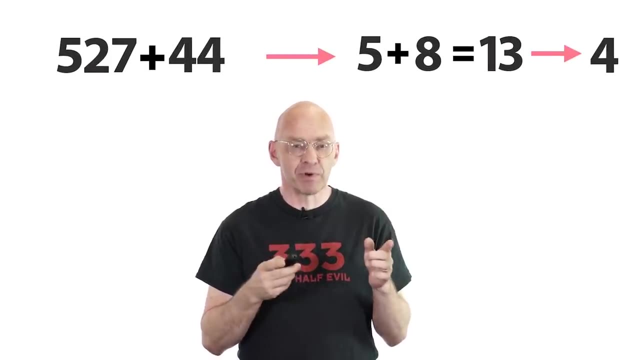 Clear Again. this is the sum shortcut. The remainder of the sum is simply the sum of the remainders or the remainder of that remainder sum. That's also good to know, right. What's even more important for us is that the same also works for products. 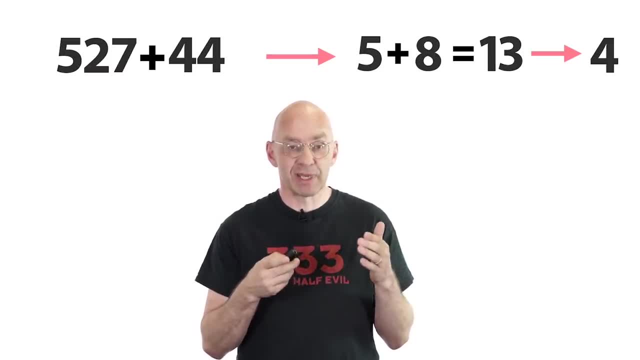 So 527 times 44 has the same remainder as 5 times 8.. 5 times 8 is 40. And when we divide 40 by 9 we are left with a remainder of 4.. So the remainder of 527 times 44, on division by 9, is 4.. 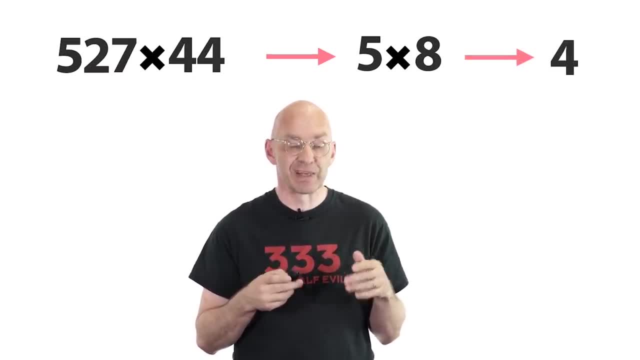 So the remainder of 527 times 44, on division by 9, is 4.. Okay, what about digital roots? Same thing, right. The digital root of the sum or product of two numbers is equal to the digital root of the sum or product of their digital roots. 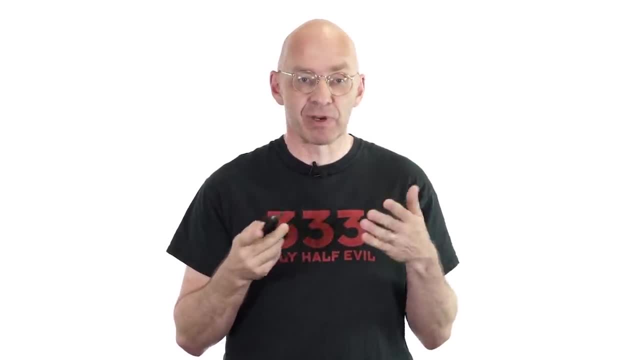 Very nifty Again to summarize, at the level of remainders, the sum and product property holds for division by any number: Division by 2,, 3,, 4,, 5,, 666, division by any number whatsoever. 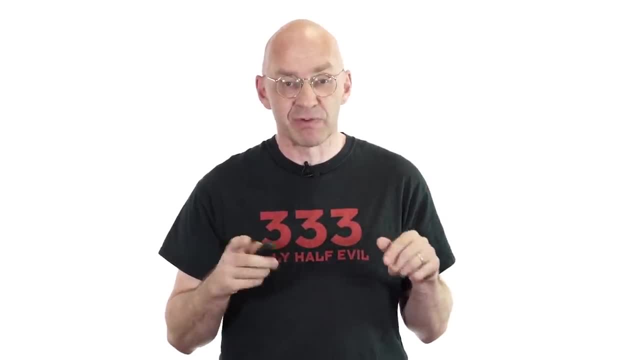 However, in the special case of division by 4, division by 9 is 4.. In the special case of division by 9 and division by 9 only, we have this extra niceness. that remainders essentially correspond to the digital roots. 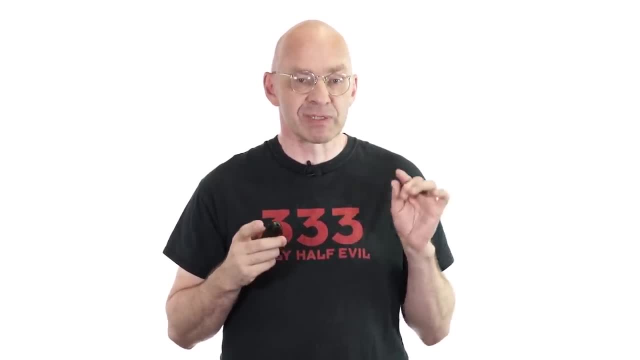 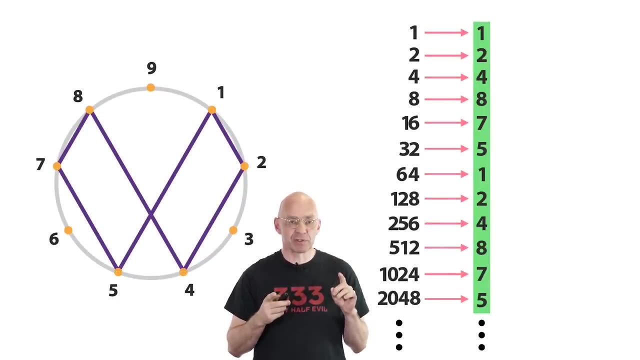 All clear. Okay, now let's use these properties to explain what's going on inside the vortex. Remember we started by looking at the sequence of powers of 2.. In other words, we kept multiplying by 2, starting with 1.. 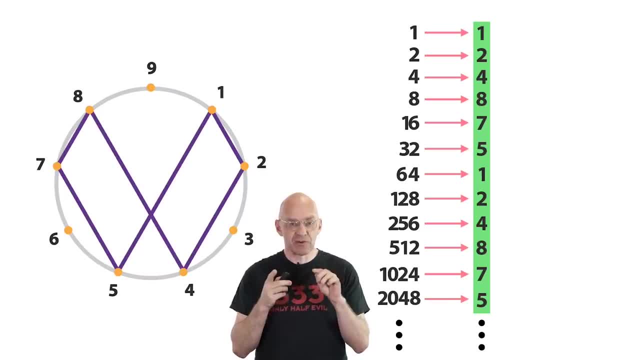 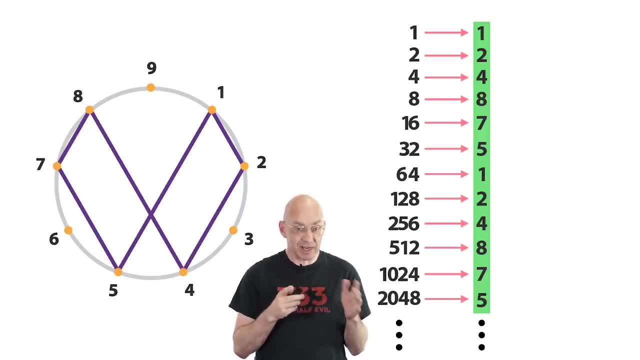 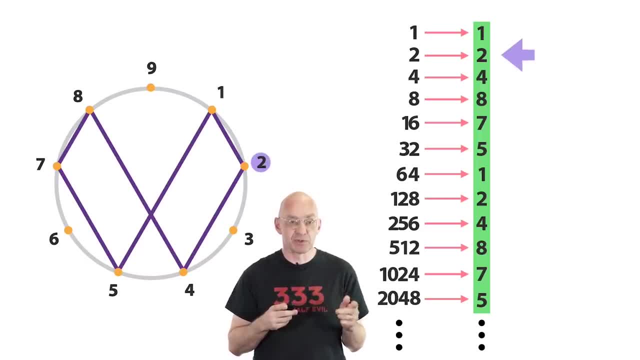 1 times 2 is 2.. 2 times 2 is 4.. 2 times 4 is 8.. 2 times 8 is 16.. And the digital root of 16 is 1 plus 6 is 7.. 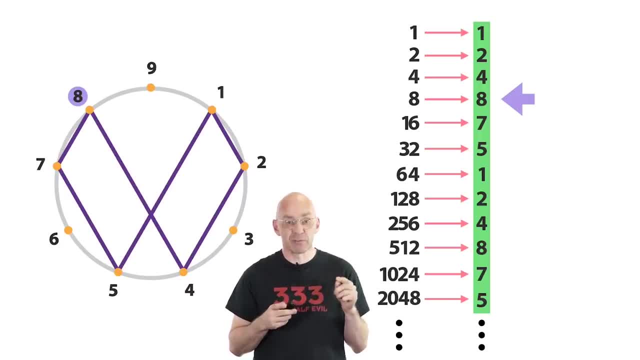 2 times 7 is 14. And 1 plus 4 is 5.. 2 times 5 is 10.. And 1 plus 0 is 1.. And so on Works, And so, looking at it this way, it's actually not such a big surprise that the numbers on 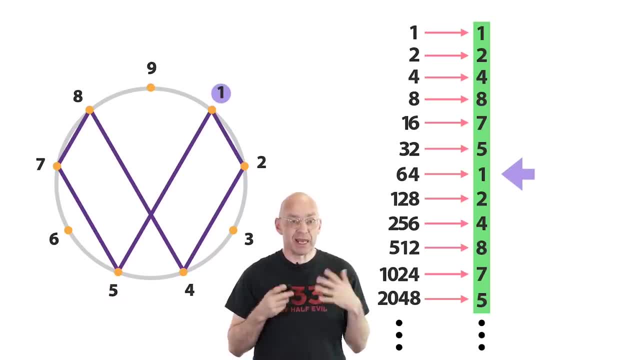 the right will eventually repeat. Why? Because the numbers on the right will repeat. Why? Because the numbers on the right will repeat. Why? Well, we are always doing the same thing over and over: Right: Multiply by 2. Followed by: find a digital root. 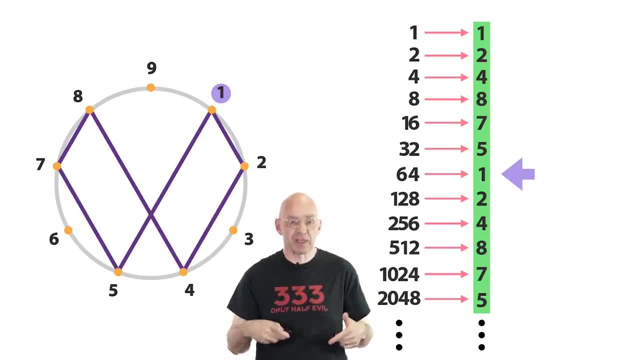 Multiply by 2. Followed by find a digital root. And since there are only 9 different possible outcomes of this operation, things are bound to repeat and then loop on forever. And of course, the same is true if we start with any number and keep doubling, and digital. 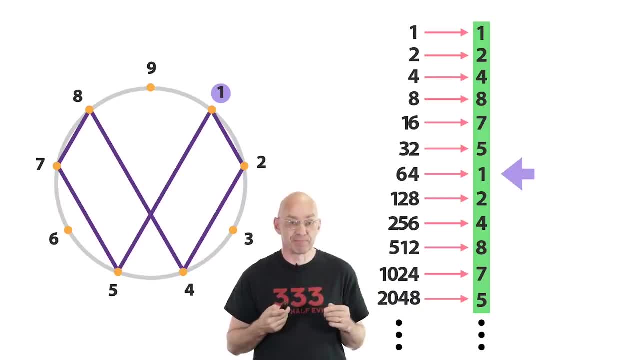 rooting, Eventually Things are bound to repeat And from there on any number goes repeated, Correct. The same is true if we start with any number and keep doubling and digital rooting, Eventually things are bound to repeat And from there on they repeat. 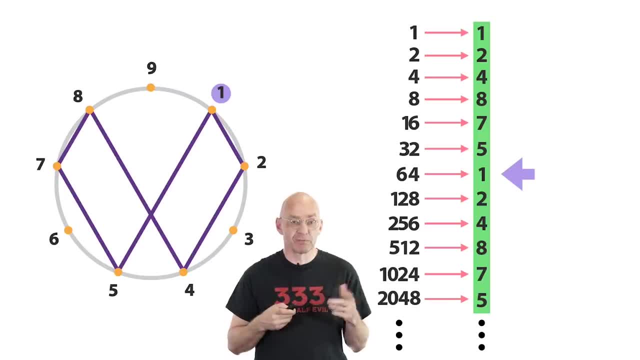 will loop forever. Starting with 3, we get a very small loop, 3, 6, 3, 6, 3, 6 and so on, And starting with 9, well, doubling keeps producing numbers divisible by 9, which all have digital root 9.. So just the miniest of mini loops in the case of 9.. 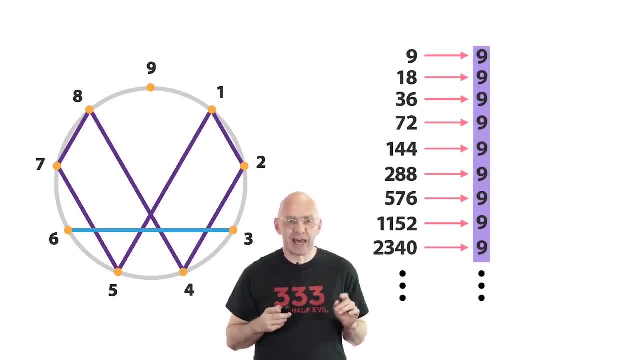 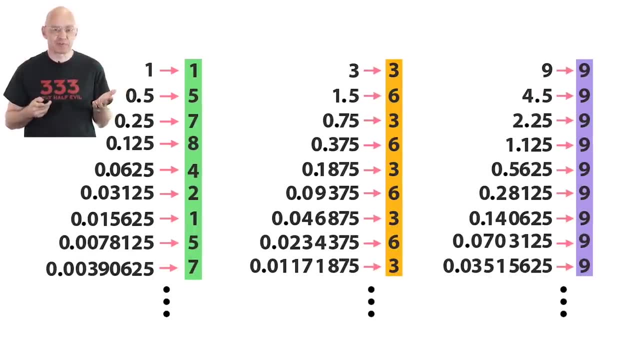 Okay, that's great. Now what about those halving sequences? They're a bit unusual and, in fact, I've never seen anybody calculate the digital roots of decimal fractions before watching these Tesla videos. Having said that, with what we know, it's also not hard to explain why we end up with the same sequences of 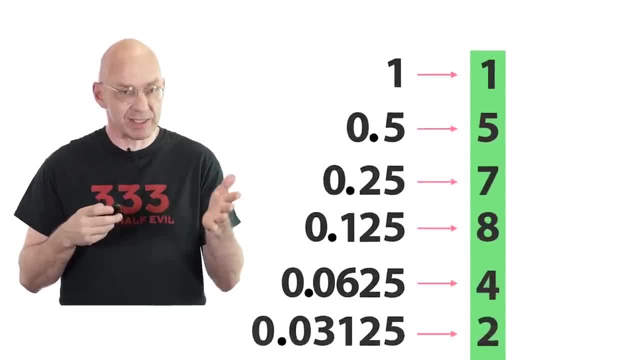 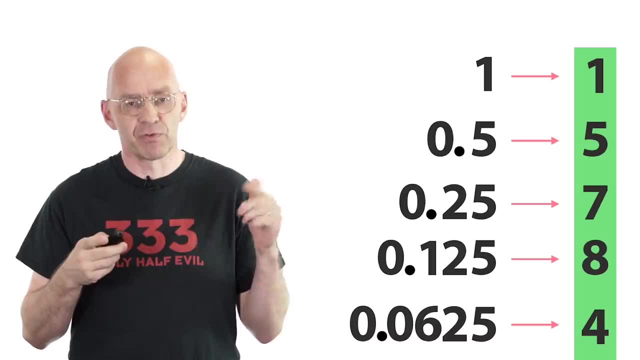 digital roots, as before, running in reverse Right To get those decimal fractions. we keep dividing by 2 to get: 1 half is equal to 0.5,, 1 fourth is equal to 0.25,, 1 eighth is equal to 0.125, and so on. Now I'm sure that you've all seen. 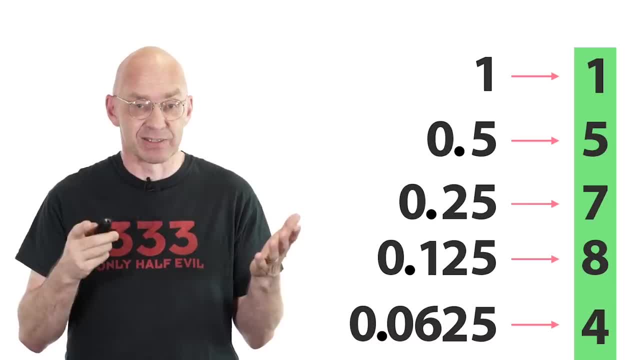 these numbers a million times? yes, but I'm sure that you've all seen these numbers a million times, yes, but did you ever notice the powers of 5 in these numbers? Wait what, Yes, powers of 5.. Just get rid of the decimal point and all the zeros and you get 5,, 25,, 125 and 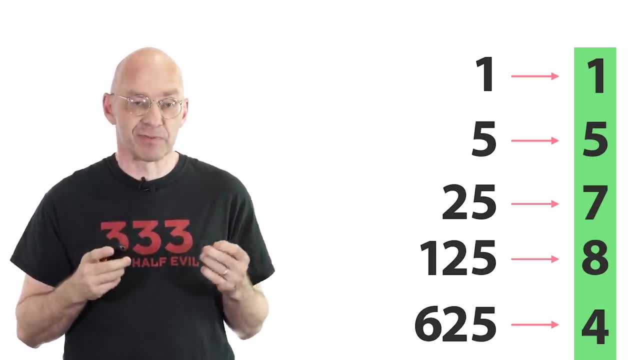 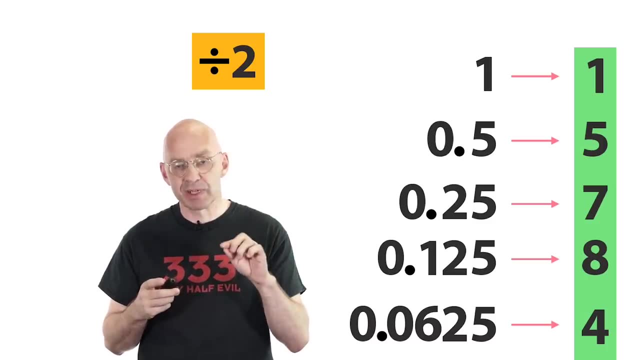 so on The powers of 5.. Where do those powers of 5 come from? Well, actually, that's also not hard to explain. You see, dividing by 2 is the same as first multiplying by 5 and then dividing by 10.. Right, 5 divided by 10, that's 1 half. 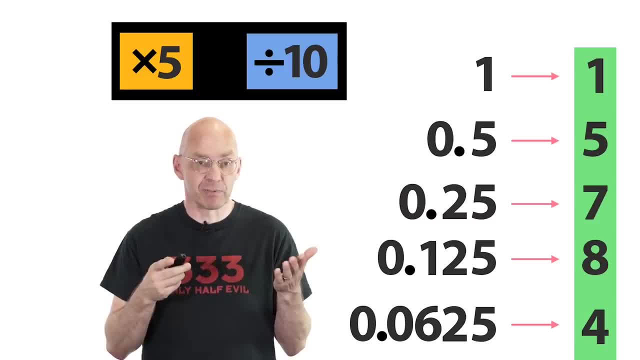 And of course, dividing by 10 only moves the decimal point. This means digit wise. we end up with the powers of 5 and a couple of zeros. Neat, eh. And now the rest I leave is a little challenge for you. Why are the digital? 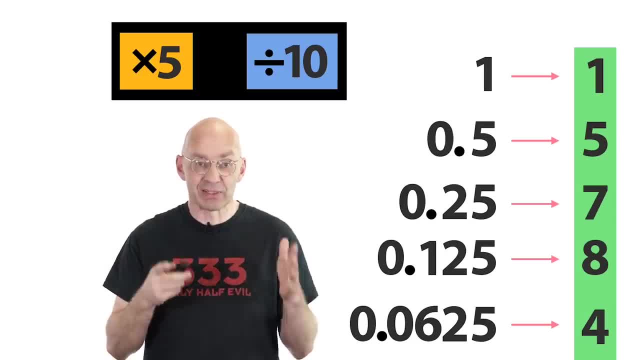 roots of the powers of 5, looping the same way as the powers of 2, just in reverse. Leave your answers in the comments. Again, the key is that 2 times 5 is equal to 10, and what's the digital root of 10?? 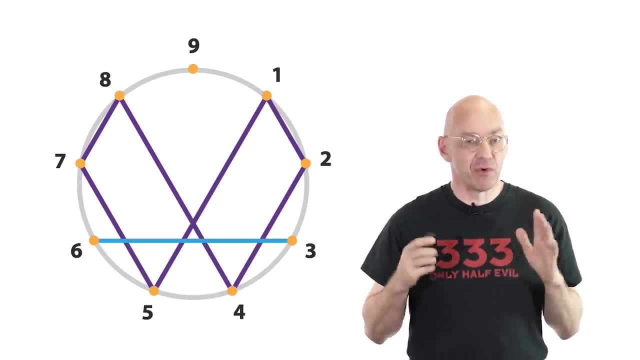 Ok, getting there. as far as mathematics is concerned, the vortex is simply a visualization of what happens when we multiply the remainders from division by 9 by the number 2.. In technical lingo, what we are doing here is multiplication by 2 modulo 9.. Actually, I 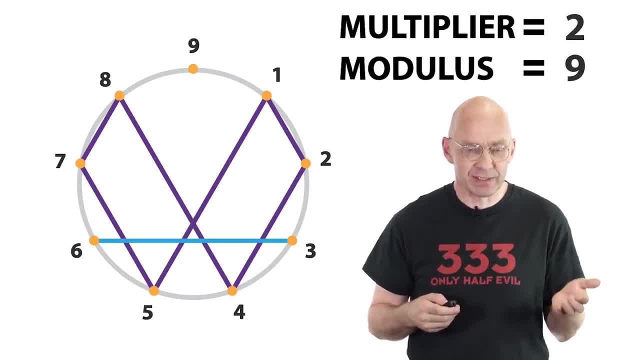 almost forgot. if we want to think of the vortex in terms of remainders and not digital roots, we should replace the 9 at the top by 0. Remember that little difference, right? And what about the other diagrams that I showed you earlier? 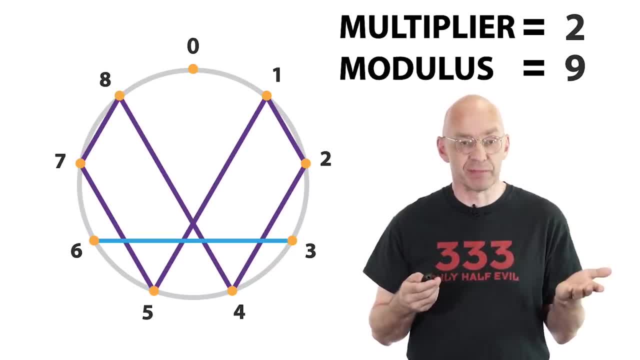 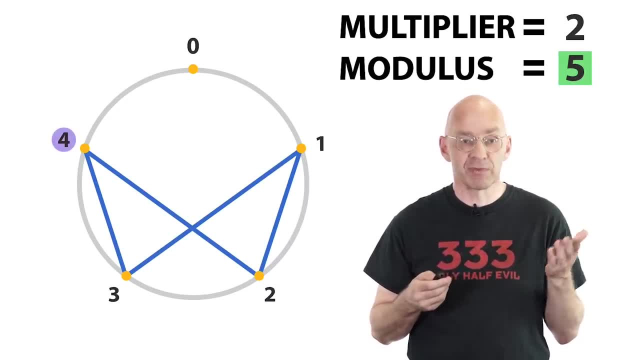 Well, those are visualizations of multiplication by 2 modulo other numbers. Here's the diagram for 5 again right? Just a quick check there: 4 times 2 equals 8, and when you divide 8 by 5 you get a remainder of 3.. Taking that 3,. 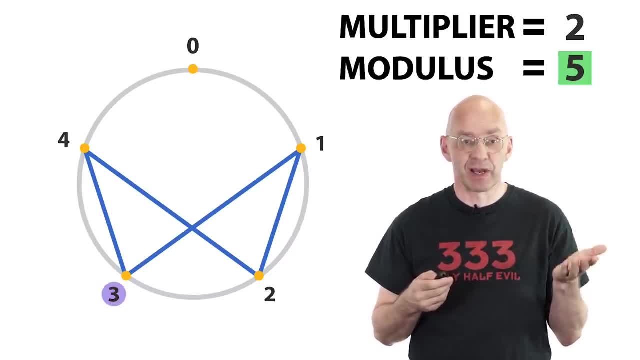 timesing it by 2 gives 6, and when we divide 6 by 5, we get a remainder of 1.. And so on Works. And then, as I already showed you before, as we erase the modulus, the number by which we divide the first real magic occurs with the 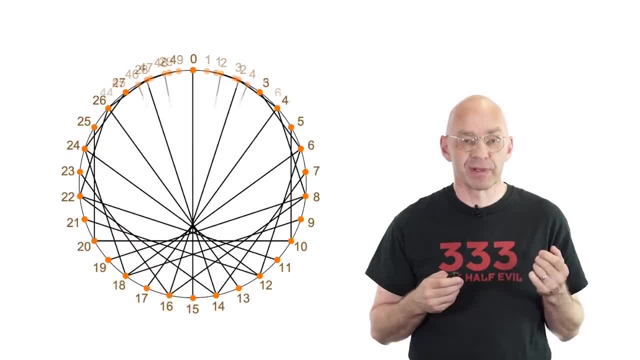 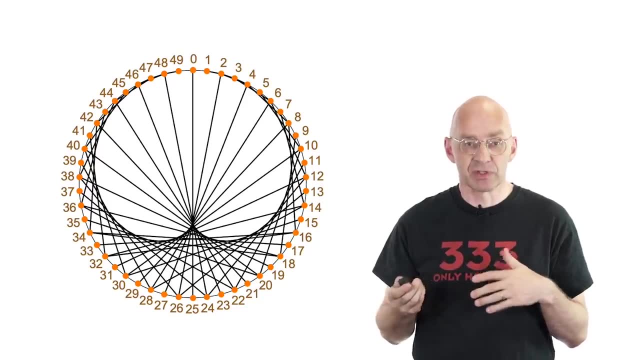 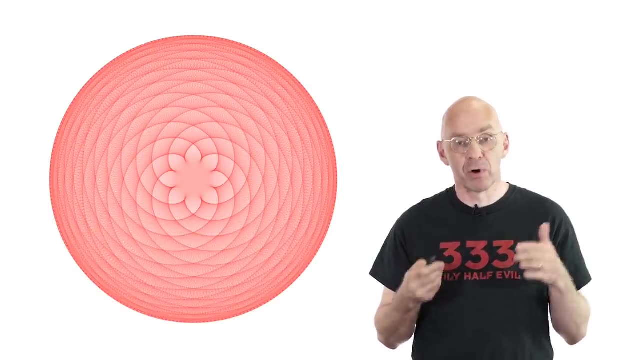 cardiot materializing out of nowhere. Very nice, But all this is really just multiplication by 2.. The other diagrams I showed you you get when you multiply by other numbers. So, for example, have a look at this crazy diagram here. This is multiplication by 240 modulo 7417.. Who? 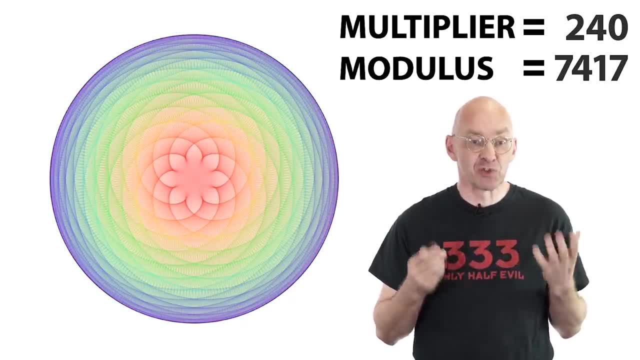 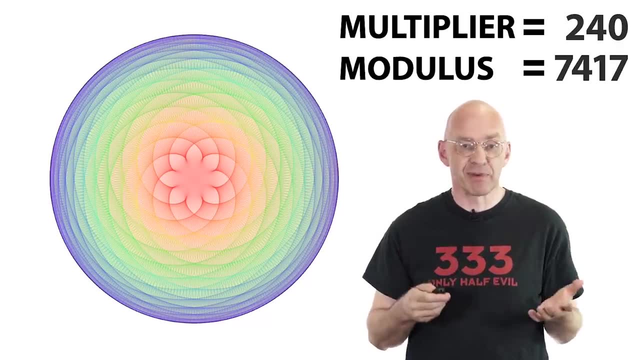 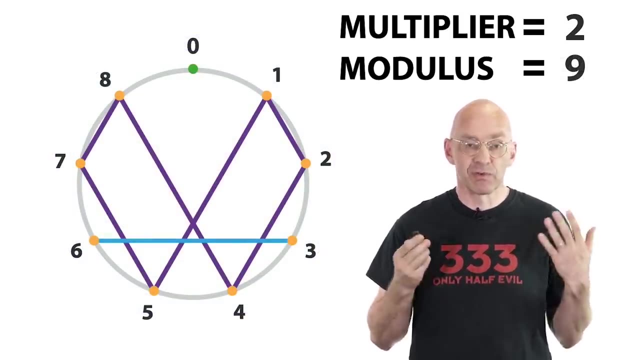 would have thought. Now, multiplication modulo different numbers is super important. mathematics, with myriads of applications within and outside of mathematics, Finite fields, cryptographic algorithms, number theory in general, and so on. In an app for drawing these diagrams, we then have two basic controls: one for setting the number we multiply with and one for 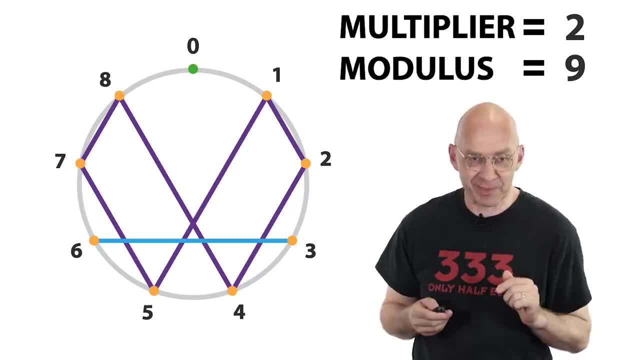 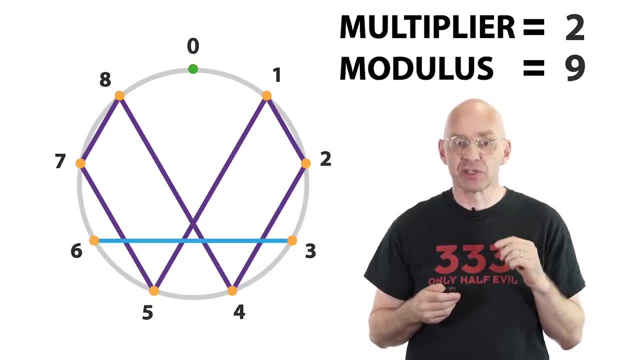 setting the modulus. In fact, let's have another coding competition. Whoever among you submits an online app that implements drawing these diagrams enters into a draw for Marty's and my new book. That one there, Anyway. for the vortex we have multiplier 2 and modulus 9, then changing the modulus to 50 and then the. 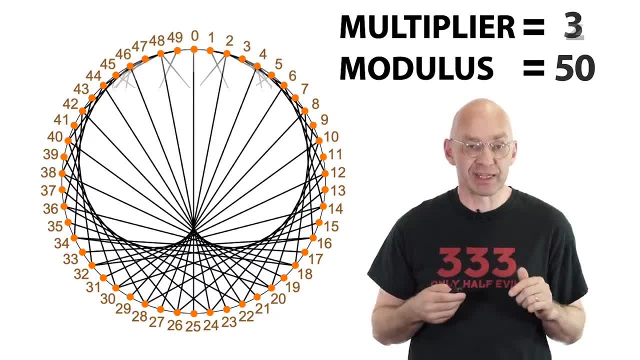 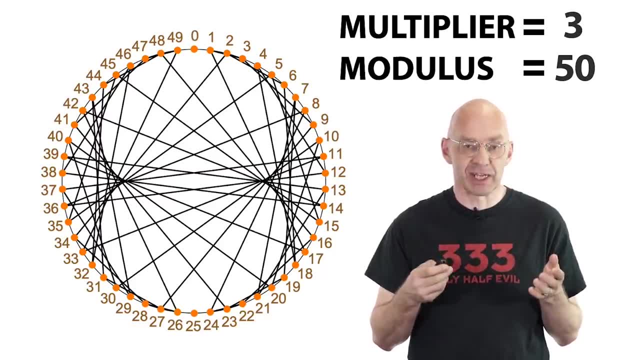 50, we get this, And if we now change the multiplier to 3, we get this. Actually, on closer inspection, there's at least one more aspect of these diagrams which we could also change. Can you guess what I've got in mind here? It's a tricky one. 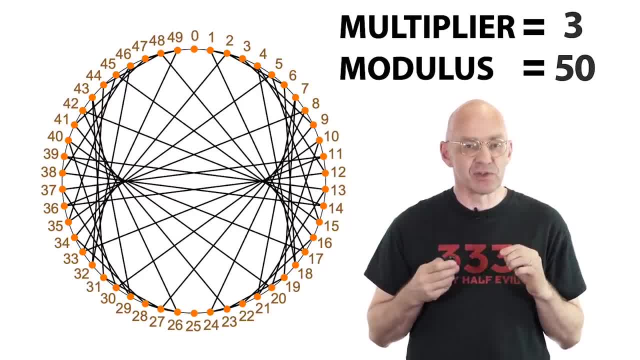 and easily overlooked. Let me give you a hint: It's got to do with the 9 occupying a special role in our discussion. so far right, Only for modulus of 9 can we use the digital root algorithm to construct these diagrams. This does not work for. 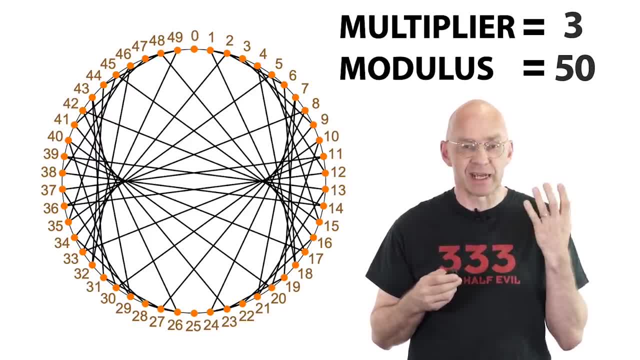 any other diagram. So what exactly is it that makes 9 special in this respect? Well, vortex mathematicians will probably tell you that 9 is special. It's just part of Tesla's 3, 6, 9 being the key to the universe. Of course 9 has to be. 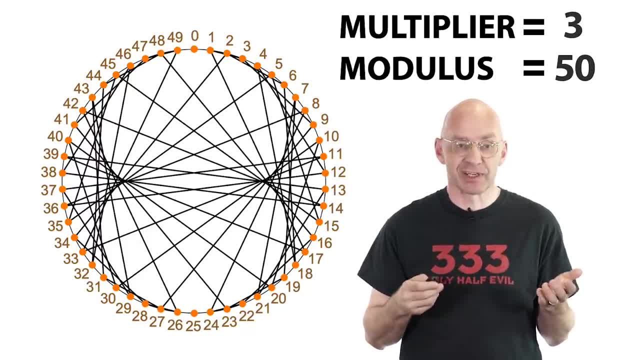 special right. Actually, on closer inspection, it turns out that, in the first instance, 9 is special because we're writing numbers in base 10.. Wait what? Yes, the visibility test for 9 and all the other digital root magic is a direct consequence of us writing numbers in. 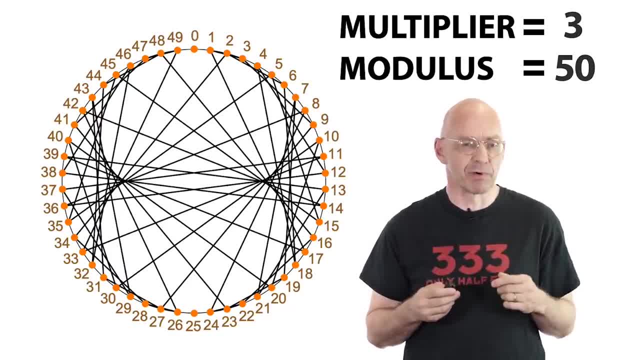 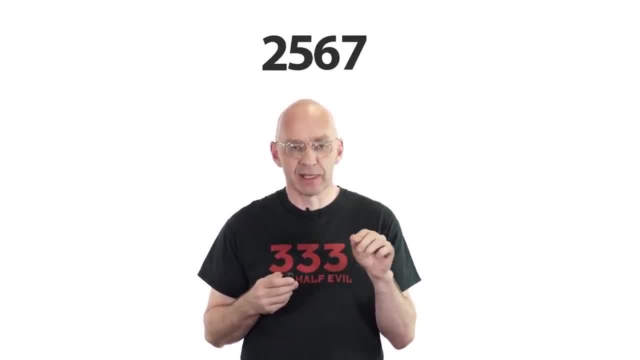 base 10.. Interesting, huh? You want proof? No problem. Let me show you why. the remainder of this number, on division by 9, is the same as the remainder of the sum of its digits. That's what makes the digital root work right. Well, 2,567 is. 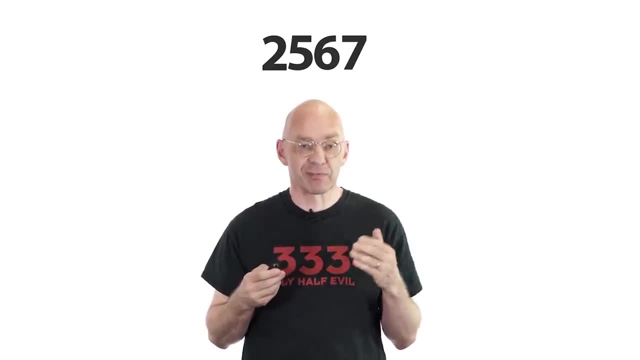 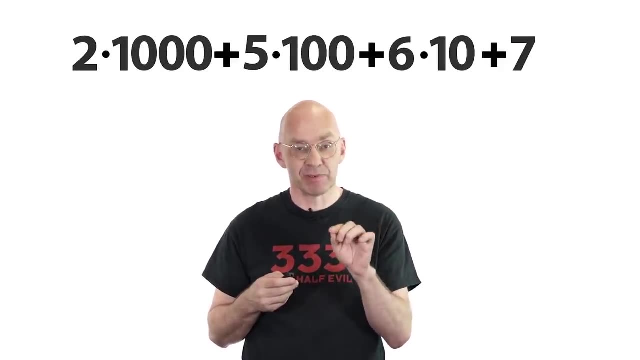 just 2 times 1,000 plus 5 times 100 plus 6 times 10 plus 7.. and 1,000 is 999 plus 1.. 100 is 99 plus 1, and 10 is 9 plus 1.. 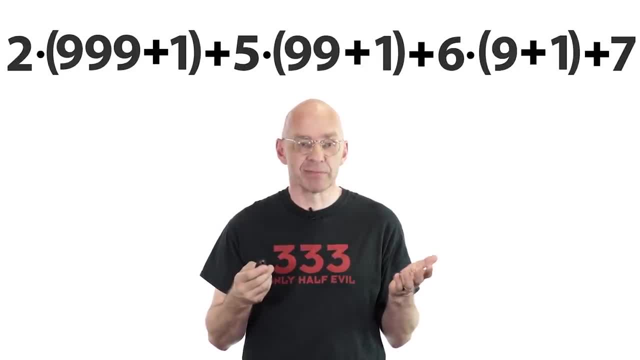 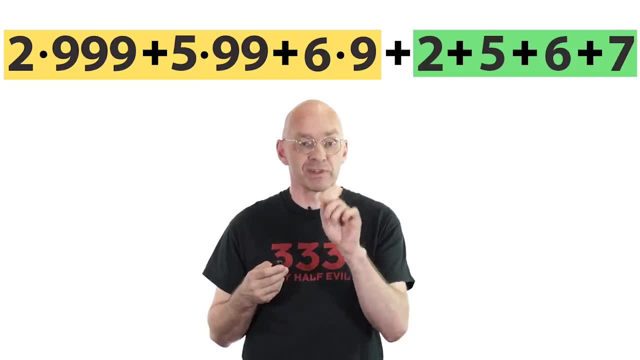 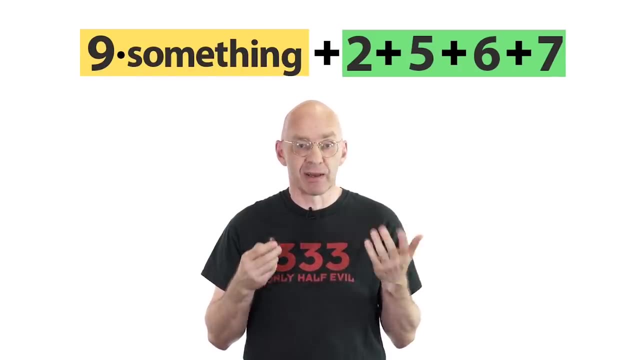 Okay, now expand and collect all the repeated nine numbers together. there Now 9,, 99, and 999 are all divisible by 9, and so the whole yellow bit is divisible by 9.. And the green bit is just the sum of the digits, and obviously the same is. 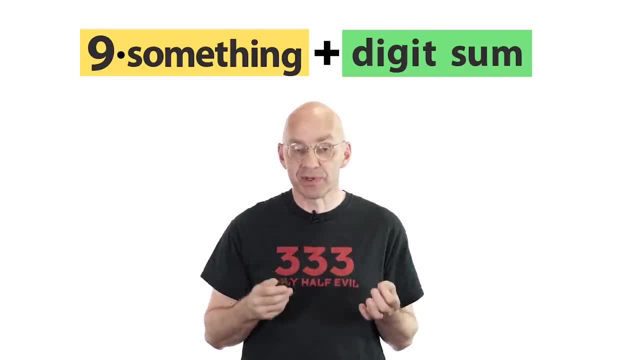 true for any integer. Any integer. integer is equal to nine times something plus its digit sum. But then, when you're interested in the remainder of the number on division by nine, we can just forget about the whole yellow bit, since it's divisible by nine, And so the remainder of our number on division by nine. 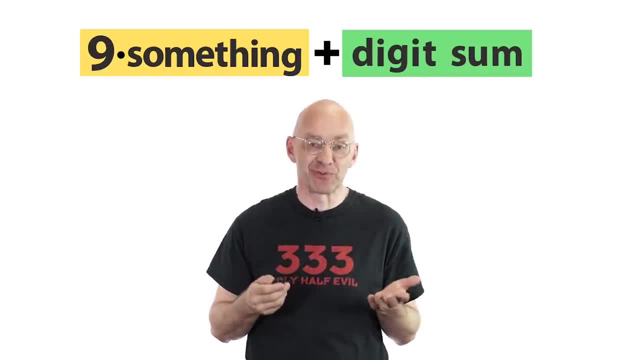 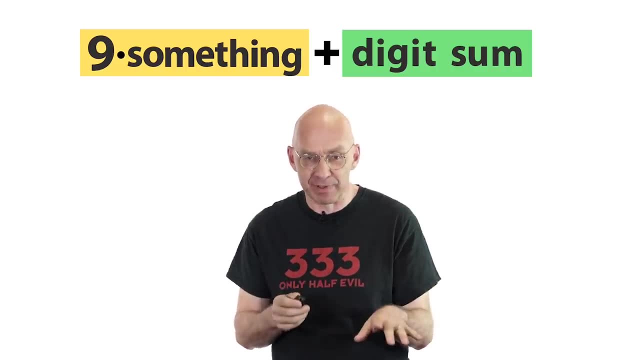 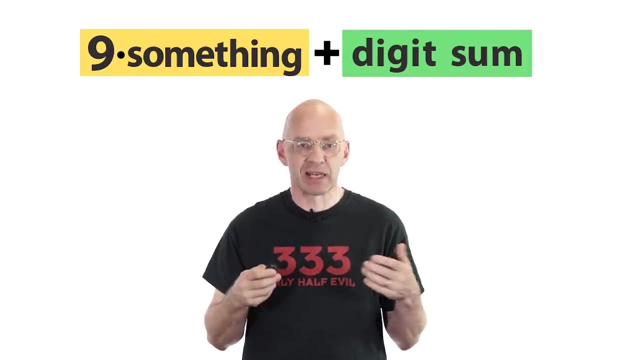 is equal to the remainder of the sum of the digits. Ta-da Proof complete, And that's why the digital sum does the trick for nine and why nine is special. Okay, but now what happens if you're an alien with b fingers and you write numbers in base b and not base 10 like we ten? 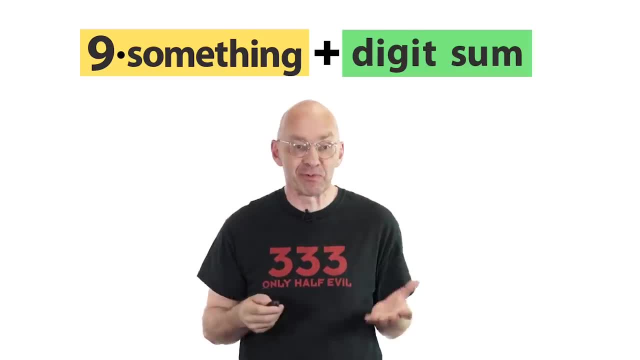 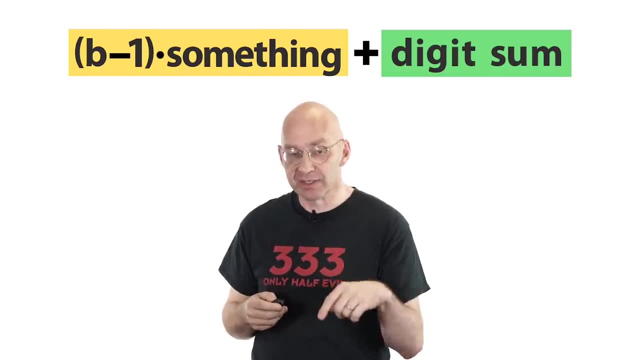 fingered earthlings. Well then, everything I said in my little proof remains true, except that nine changes to b minus one and b minus one becomes the special number. In turn, the times two diagram for b minus one becomes the special vortex diagram for an alien tesla. It's now this new diagram that can 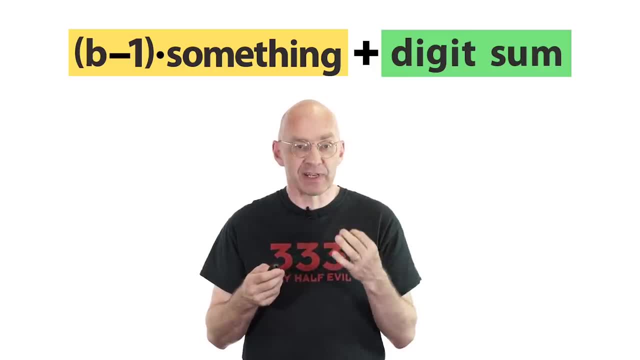 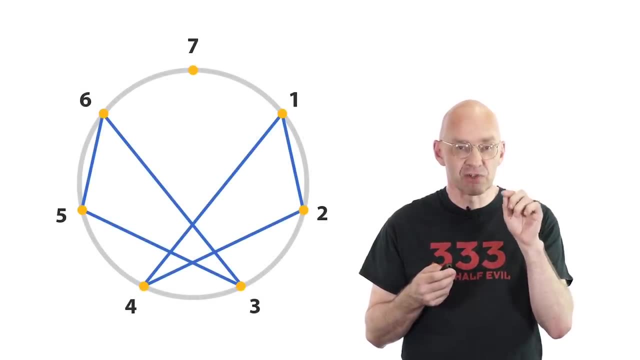 be constructed using digital roots, For example for the eight fingered tesla. we have this vortex And you can check that the digital root in base eight gives exactly these connections. For example, starting with the four, we calculate two times four is eight, Eight in. 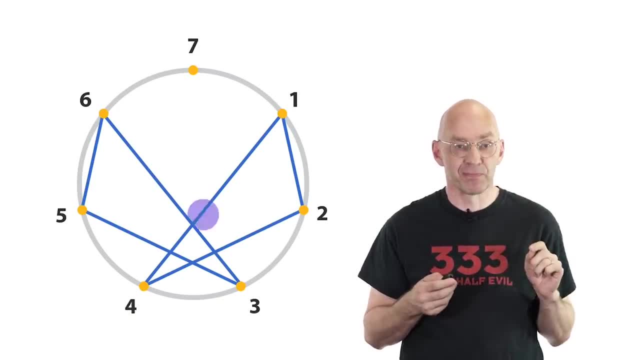 base eight is one zero, and one plus zero is one Another example. starting with five, two times five is ten. In base eight, ten is one two, and one plus two is three, And so on. Okay, so, at least from a 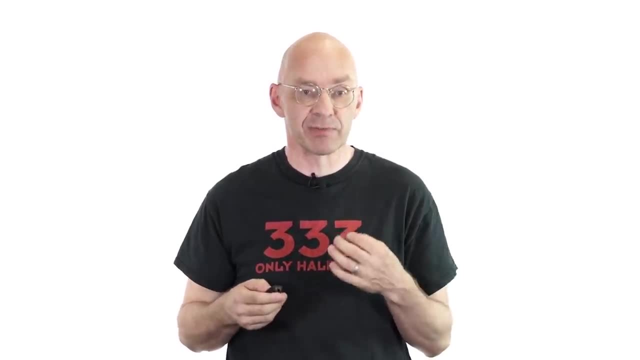 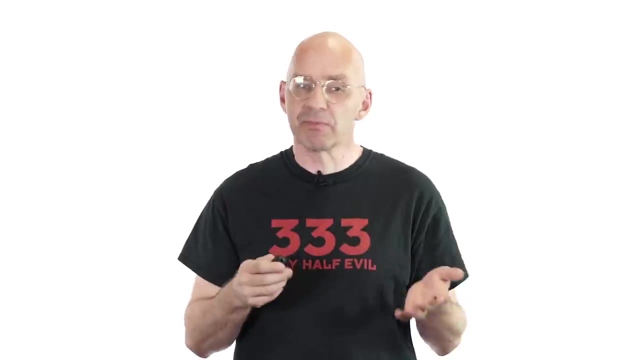 point of view, the vortex is really not that special. It's really just one of infinitely many diagrams that pretty much do the same thing And definitely, as we've already seen, many of the diagrams with large modules are a lot more spectacular from a purely aesthetic point of view. 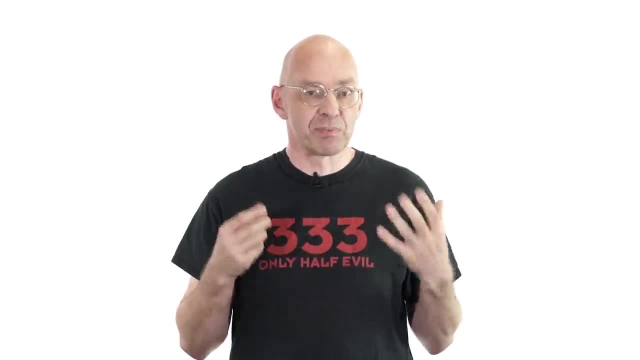 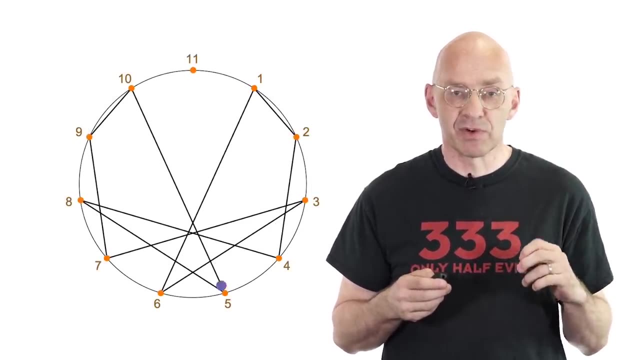 Also even mathematically. there are lots of diagrams that are superior to the vortex in many ways. For example, have a look at the diagram for eleven. In this diagram, the powers of two create a loop that is as large as possible, containing all the numbers except for eleven. Yes, 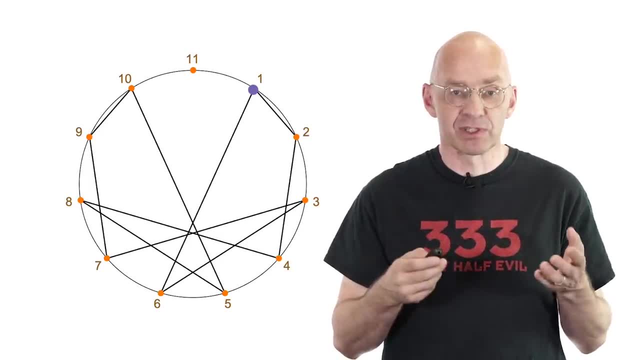 that is one continuous loop, unlike in the vortex, which consists of two loops. That such a maximal loop exists has to do with the fact that eleven is a prime number and that two is a so-called primitive element modulo, this prime. If you're familiar with these terms, you'll also recognize 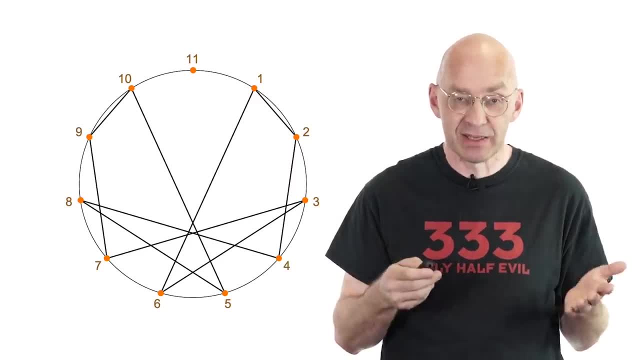 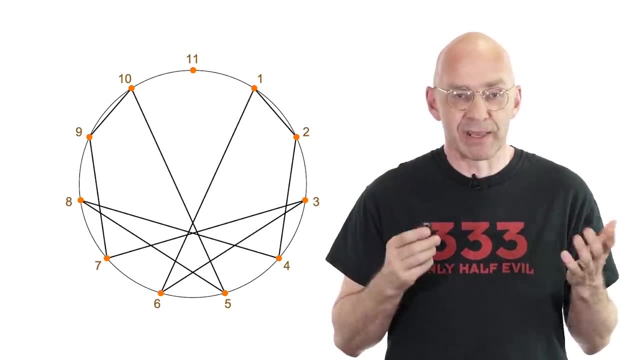 that these loops illustrate the fact that, for a prime number, p, the finite field zp has a cyclic multiplicative group, a fact which is of huge importance in mathematics. Okay, so what about the claim that the vortex is the key to a prime number? Well, the claim that the vortex is the 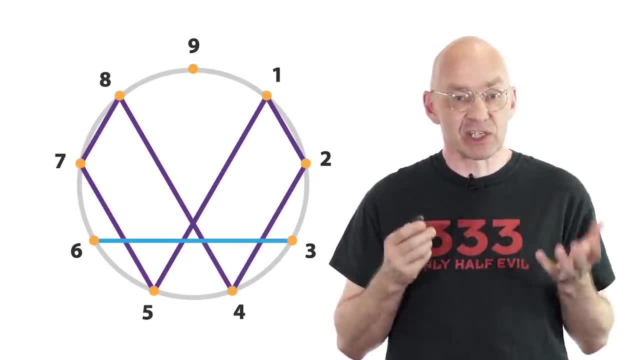 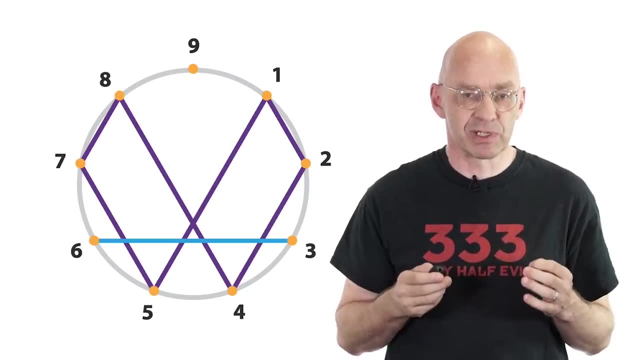 key to the understanding of the universe. Well, today's discussion was really about presenting a sound explanation of the mathematics that comes with the vortex, an explanation that demystifies its supposedly super-special properties. I hope that by now it's clear that the vortex is really. 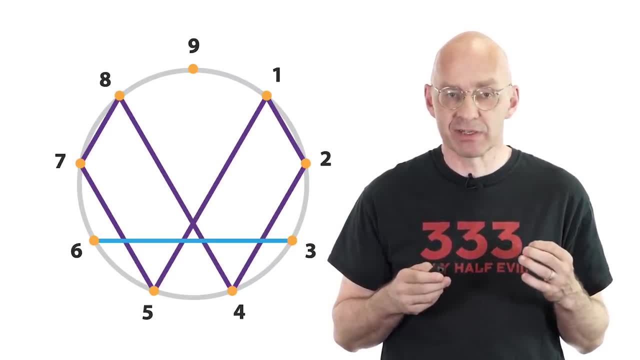 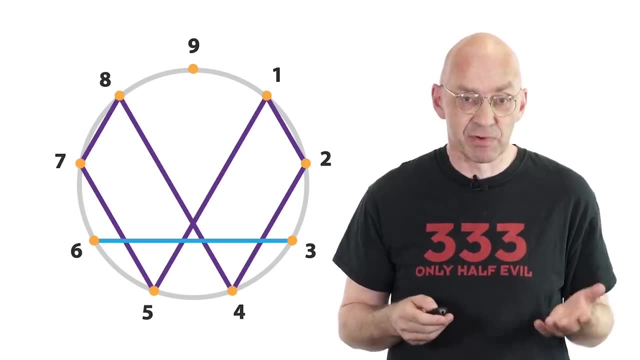 not as special and amazing as it is made out to be by all those Tesla videos, and that proclaiming it to be the key to the universe mainly based on these properties is simply ridiculous. But of course, you knew that already, didn't you? In fact, I wonder what you now think. 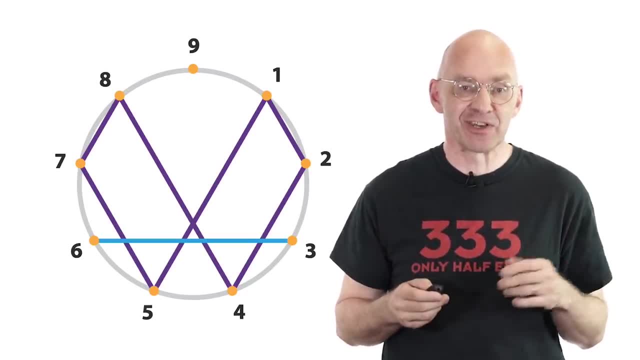 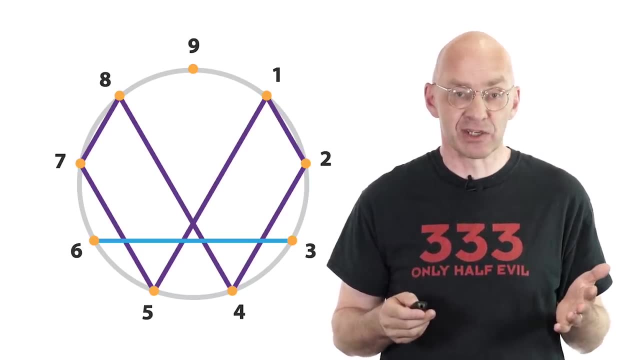 of all those Tesla videos and their creators. Please share your thoughts in the comments. Having said that, I'm convinced that mathematics as a whole is the master key to understanding the universe And, of course, the maths we talked about today is a part, a tiny, tiny part, of that key. 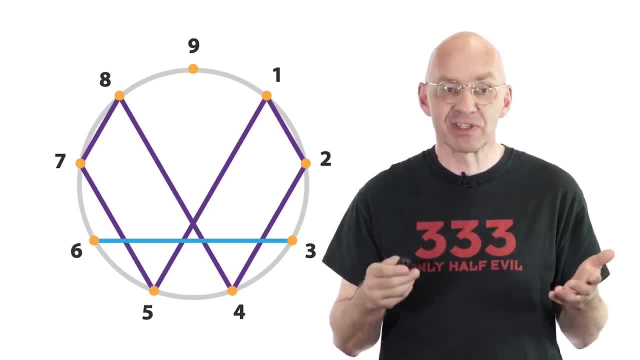 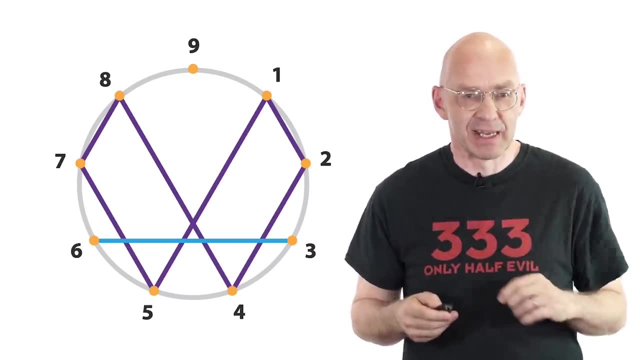 And if you're fascinated by that tiny, tiny part and are interested in a real understanding of the universe, well then, simply familiarize yourself with more and deeper maths. Okay, here's a nice challenge for you, suggested by Tristan. Take one of these diagrams. let's see if you can do it. Let's. 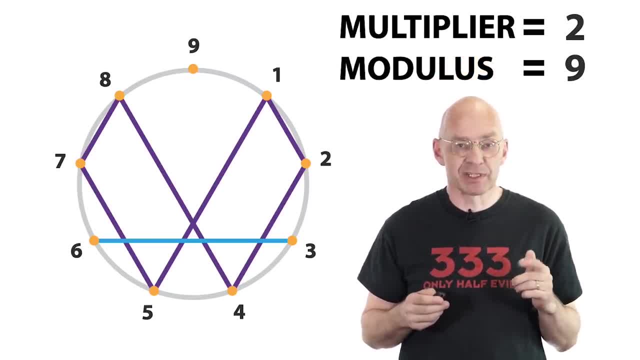 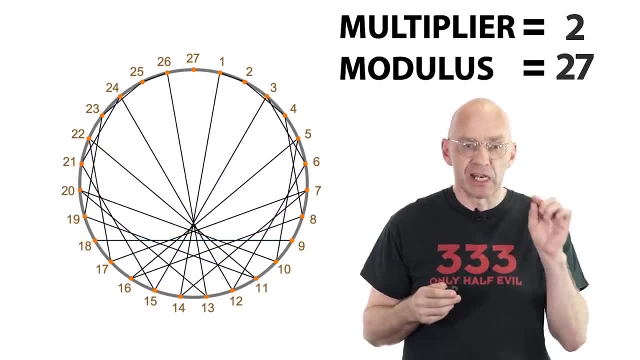 just stick with the vortex. Multiply the modulus by some integers. Say, let's multiply the vortex modulus 9 by 3, that gives 27.. Draw the new diagram. Then the loops of the first diagram are contained in the new diagram. Let me show you in this example, There, the infinity-shaped loop. 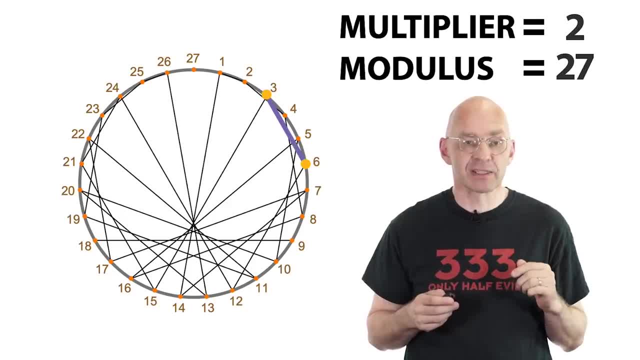 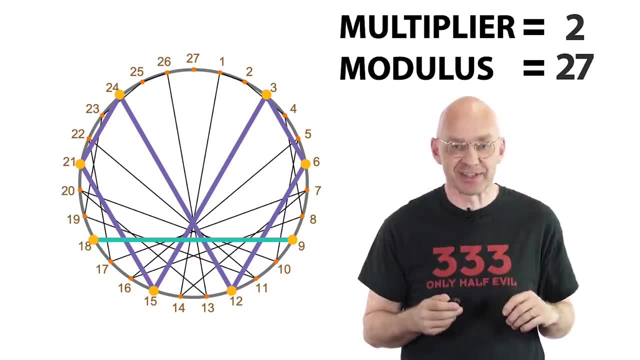 and the horizontal mini-loop of the vortex. hiding inside this diagram, There's the infinity-shaped loop and there's the other one, Whoa, super vortex, super key to the universe. Anyway, can you explain why our diagrams have this mysterious modulus multiplication property? 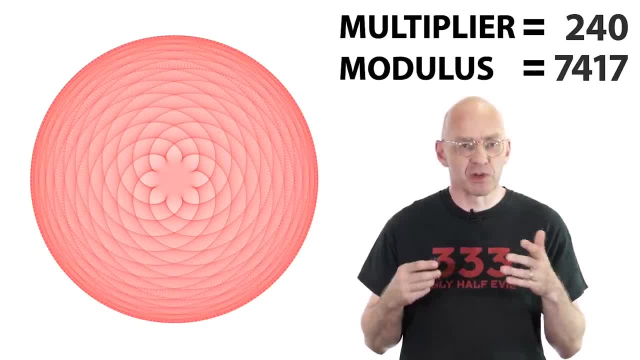 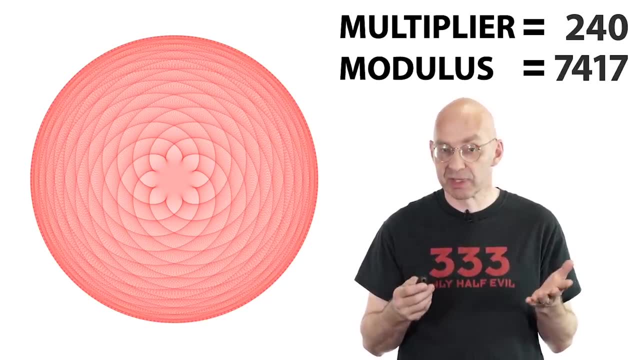 What about all these other spectacular model times tables? What is known about the crazy structures inside them? Actually, I've not been able to find much about these diagrams in the mathematical literature. Maybe some of the pros among you can do something about this sorry state. 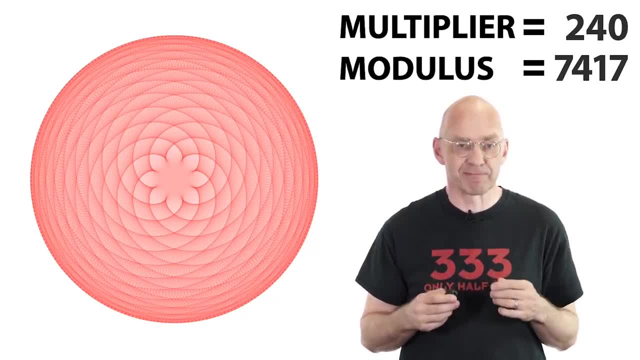 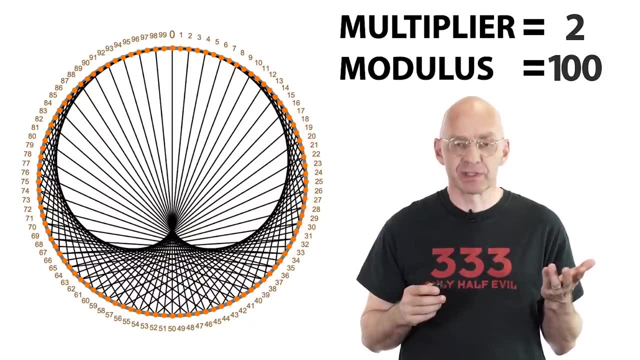 of affairs and fill in the gaps in our knowledge In this respect. I know of proofs that the curve that materialized in the times two diagrams is really the cardioid. This appears to be due to the famous 19th century Italian mathematician Luigi. 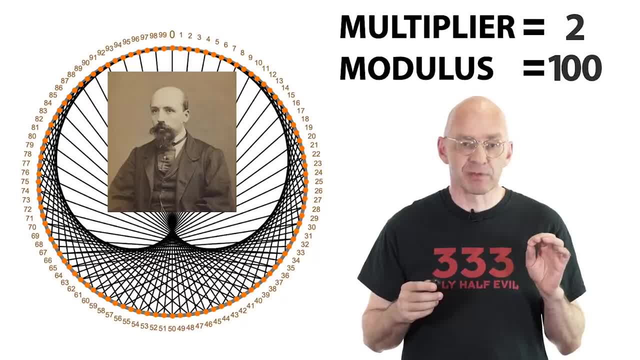 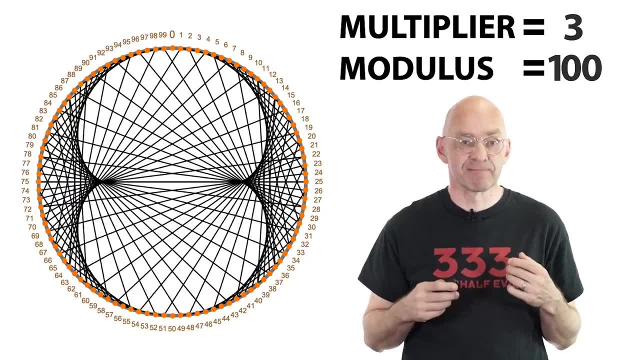 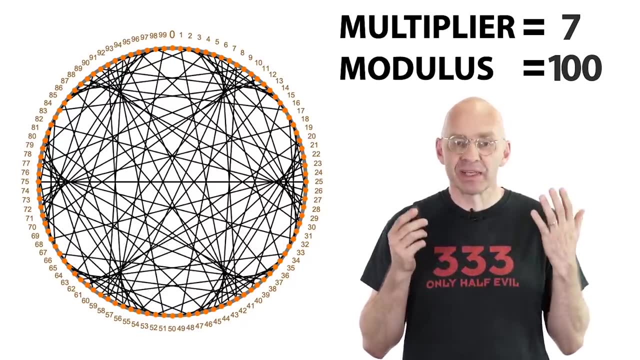 Cremona. Also, when you experiment a little with small multipliers- 2,, 3,, 4,, 5,, 6,- and large modulus, another striking pattern jumps out at us. Can you see the pattern? I'm sure you can. Why do these petals appear and why is it always one fewer? 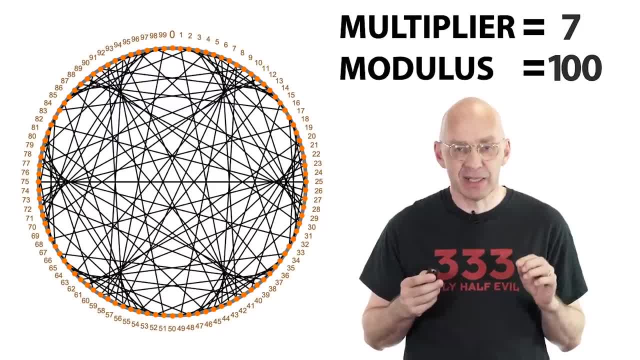 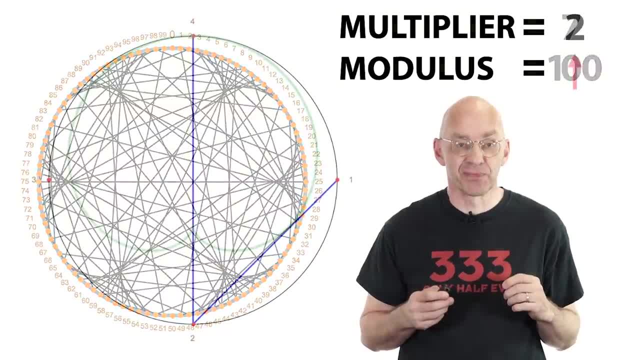 petals than the multiplier. Well, the details are messy, but it's possible to gain some intuition for the one fewer than the multiplier bit. Have a look at this animation. This is just the base case where we multiply by two. that produces the cardioid, What I'm doing. 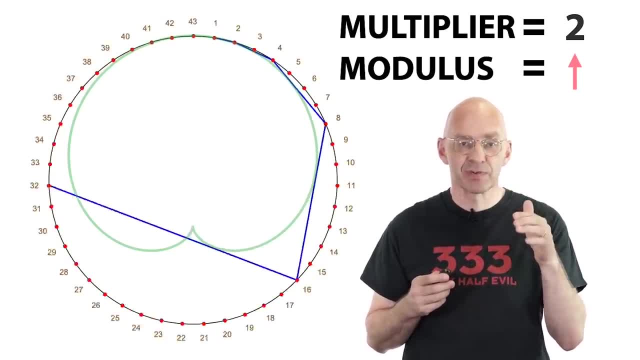 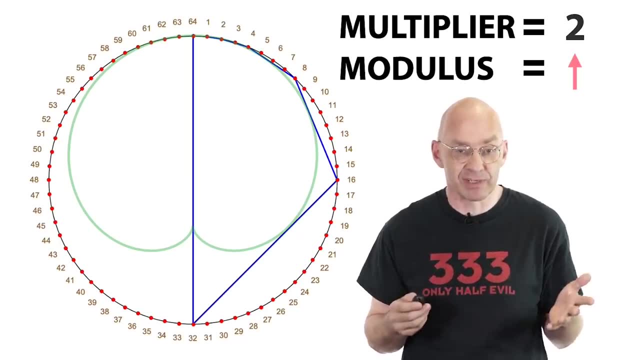 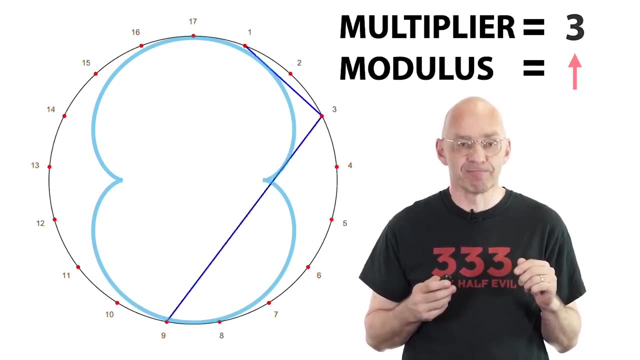 here is raising the modulus while at the same time tracing the powers of two that fit in the circle. Notice that the cusp occurs where the last connection goes straight across. Makes sense, right. Here's what happens when we set the multiplier to three. The first cusp occurs at the point x, such that three times x is ideally on the. 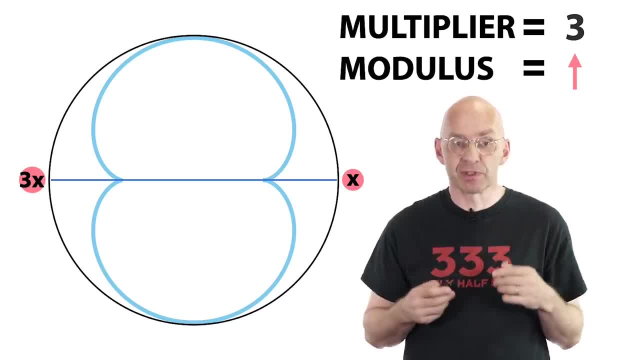 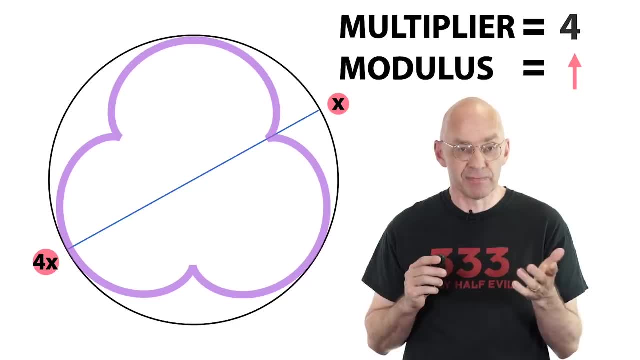 opposite side of the circle. For the next multiplier four, this picture would look like this: Now, 4 x minus x- that's the distance between the two points- is half the circle. Now we just follow our nose and solve for x. There we go Of. 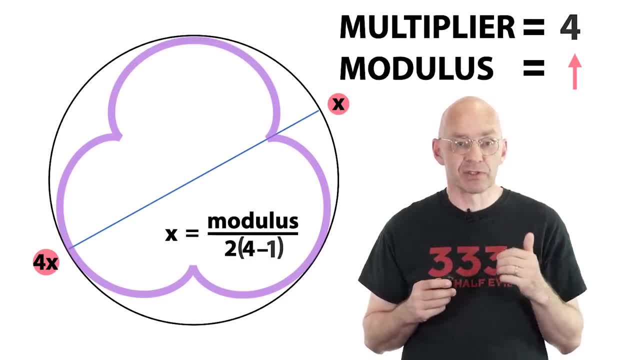 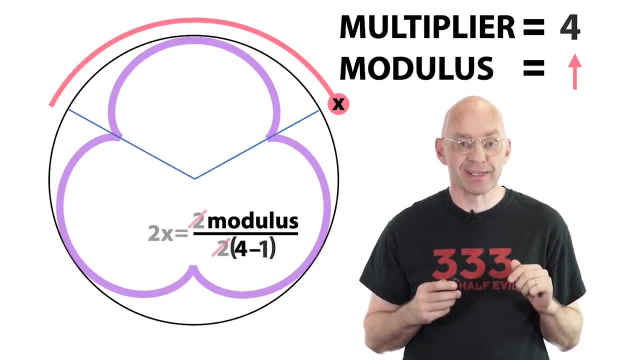 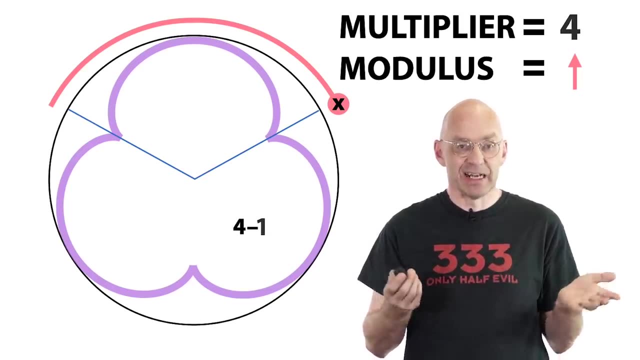 Of course, x is really just the distance from the top around the circle, and so the width of a flower petal is 2 times x, And that means that there will be a total of 4 minus 1 equals 3 petals around the circle. Tada, The same. 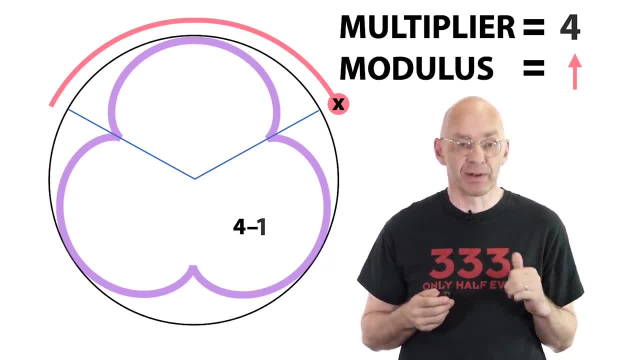 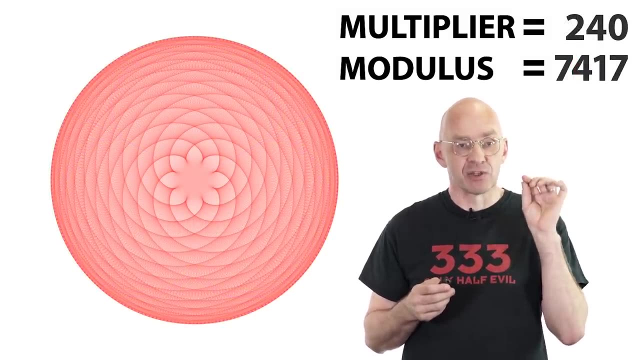 calculation shows that in general, we'll have multiplier minus 1 petals. Of course, there are still quite a few details missing from this argument to make it into a complete proof. Anyway, good enough for this video. What do you think Now? even in this monster diagram with multiplier 240, there are 240 minus 1. 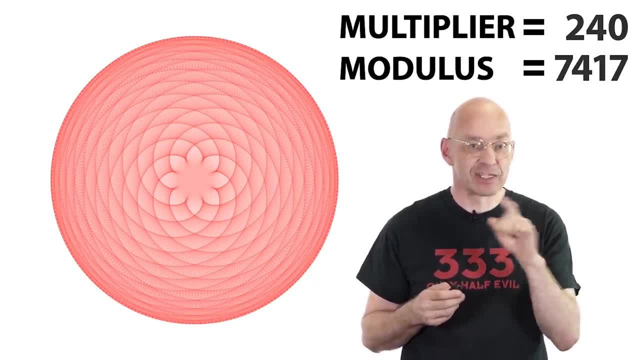 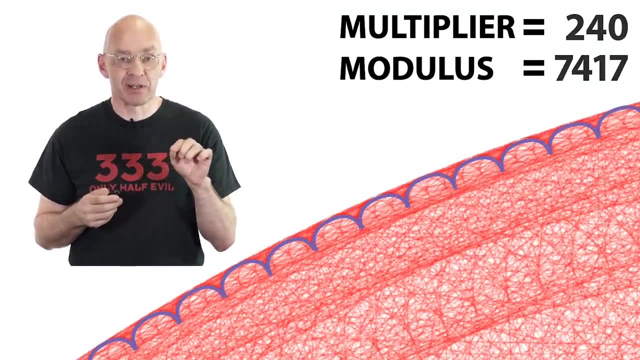 that's 239 tiny little petals around the outer circle. Let's zoom in on part of the circle. there There are lots and lots of little petals. But can you see, even at the border there's a lot more stuff going on. For example, how about this ring? 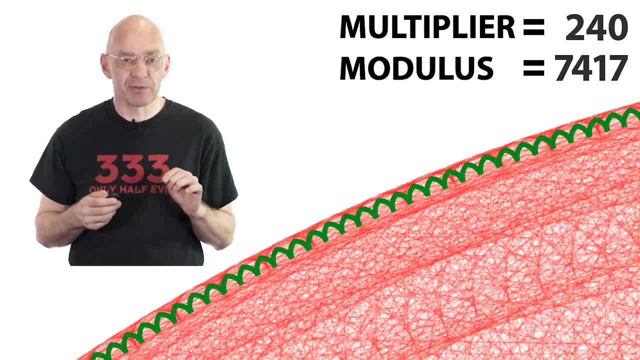 of smaller petals. Challenge for the keen among you: How many of those little petals are there and how many loops does this monster diagram have? Okay, Okay, Okay. Who can find the answers to these questions? But of course, zooming out, that's where the real spectacular stuff is happening. How exactly is all this? 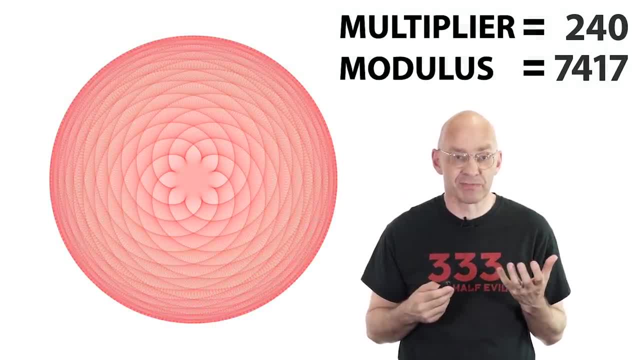 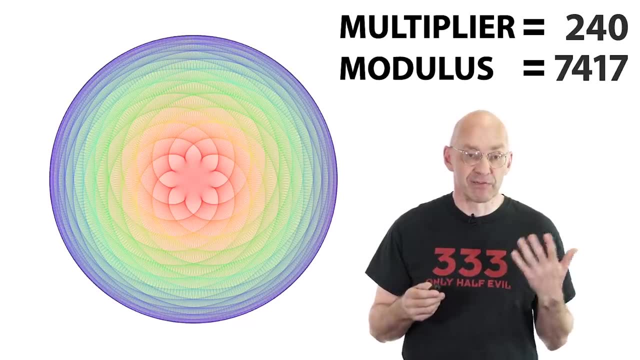 complicated and beautiful structure linked to the multiplier and the modulus. The only place I know that makes some progress towards answering this question is an unpublished write-up by Simon Plouffe that I've linked to in the comments. You may know Simon Plouffe for his involvement in the establishment of 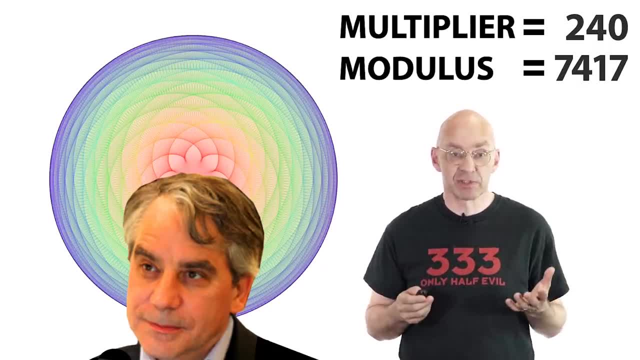 the Encyclopedia of Integer Sequences, as the creator of the inverse symbolic calculator And the discovery of the spectacular Bailey-Borwein-Plouffe formula for calculating individual digits of pi. Anyway, challenge for the super keen and capable mathematicians among you: Check out Simon Plouffe's write-up and then go where no one has gone before and 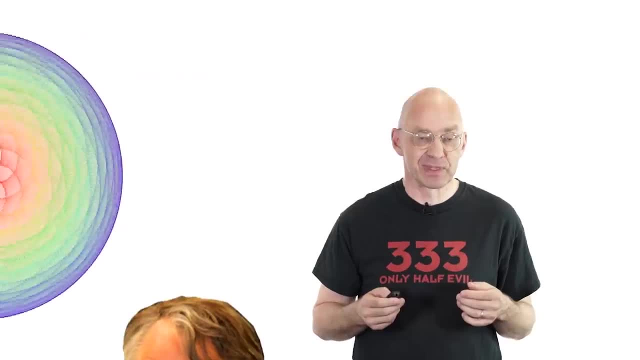 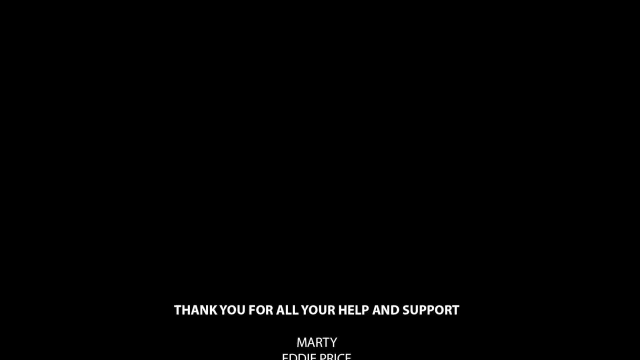 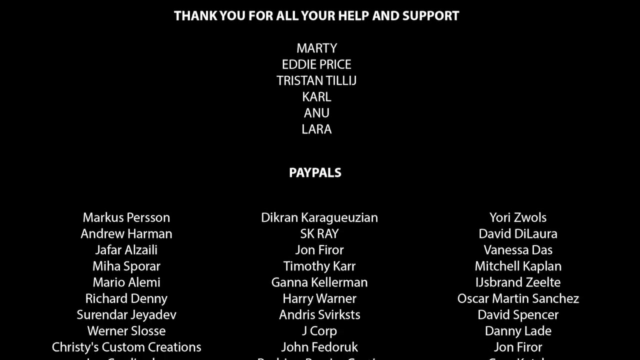 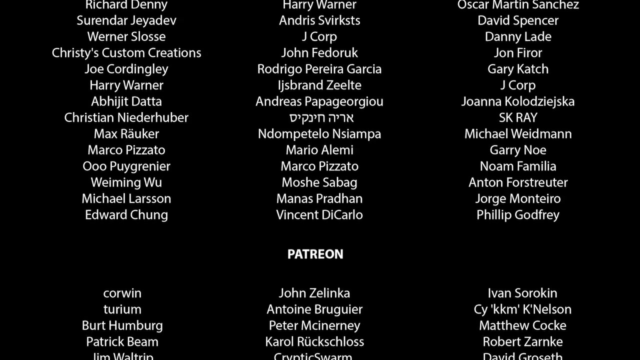 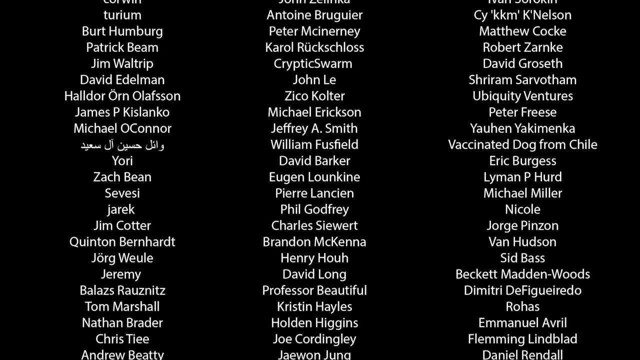 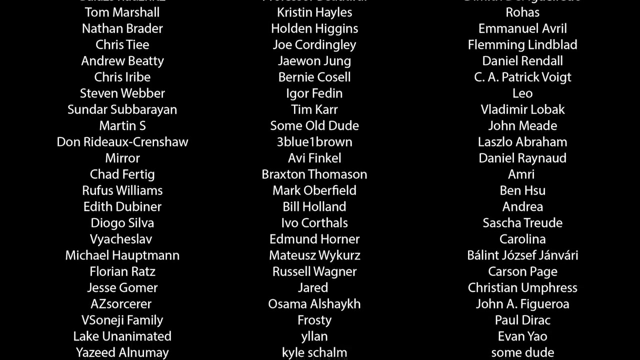 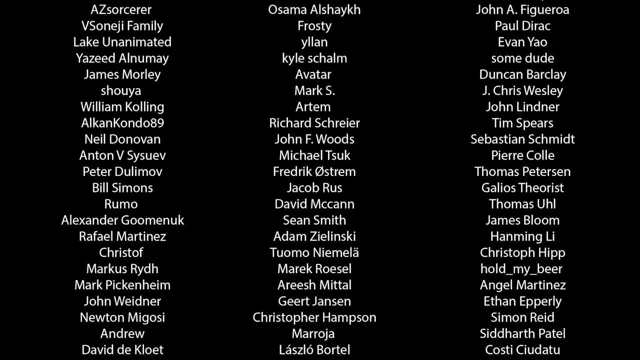 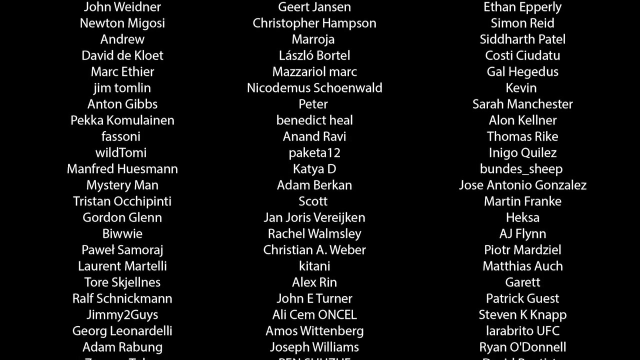 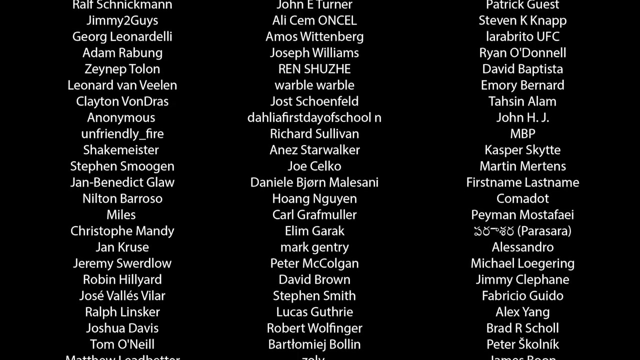 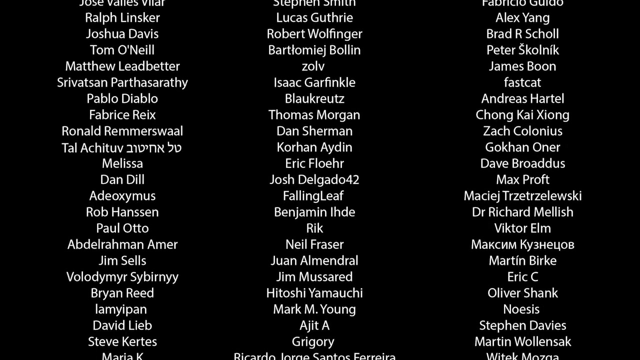 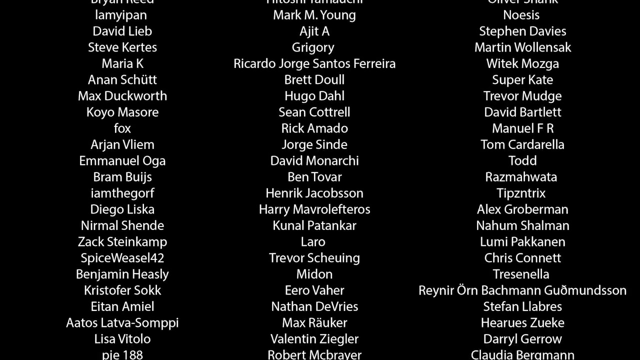 explore the secrets of these diagrams, And that's all for today. I hope you enjoyed our vortex adventure Until next time. Captions by GetTranscribedcom. Captions by GetTranscribedcom. Captions by GetTranscribedcom.